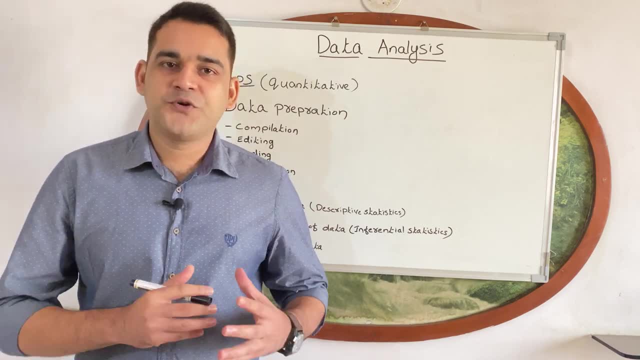 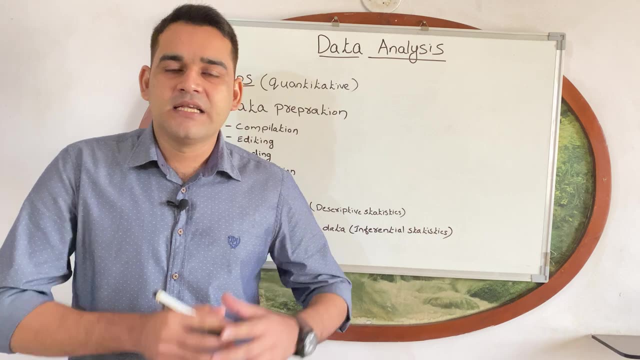 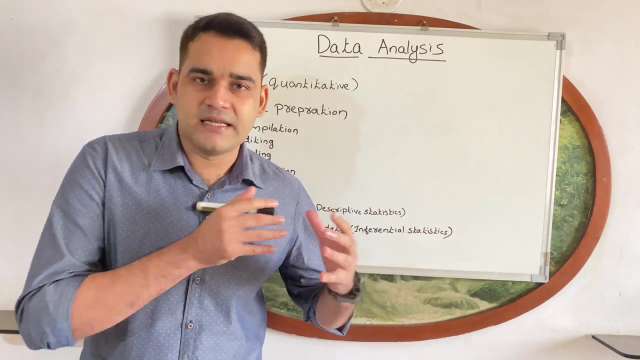 Hi everybody, I'm Naufal. Welcome to my channel. Today we are going to discuss regarding a very interesting topic, that is, data analysis, Analysis of the data and the steps of data analysis in quantitative study. So what is mean by data analysis In research? you are collecting the 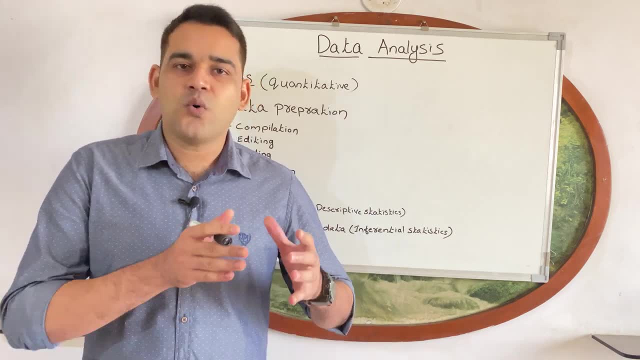 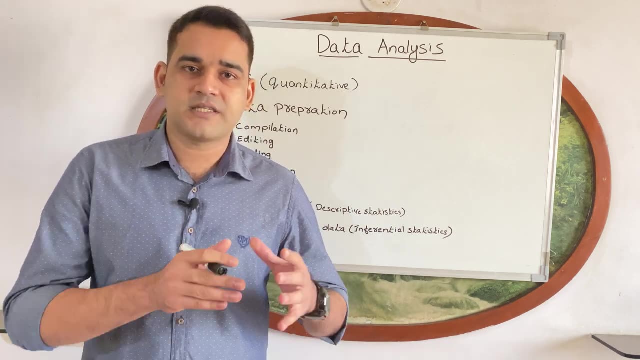 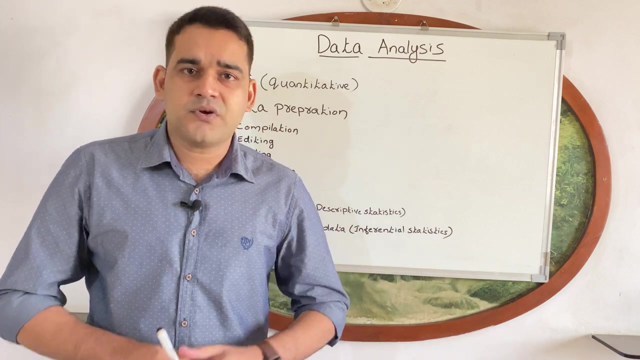 data using different methods, That is, through interview or through observation or through questionnaire. you are collecting the data. For example, a teacher want to collect the data from the students, So she is conducting an exam. So to conduct the exam, a question paper is required. 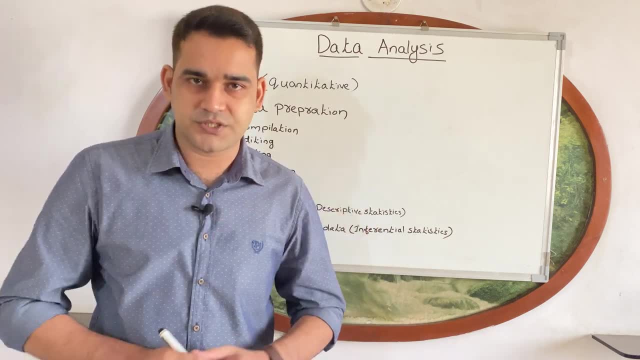 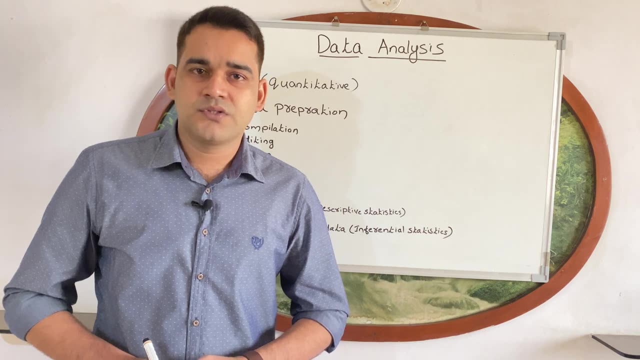 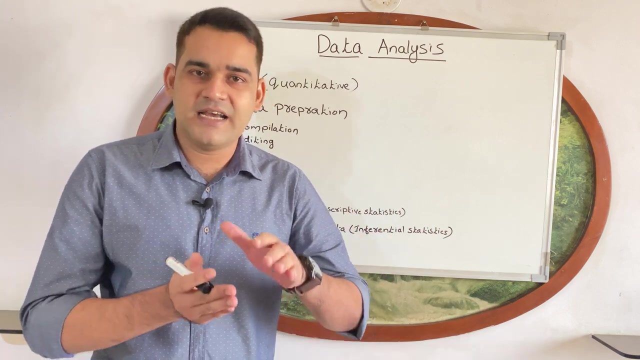 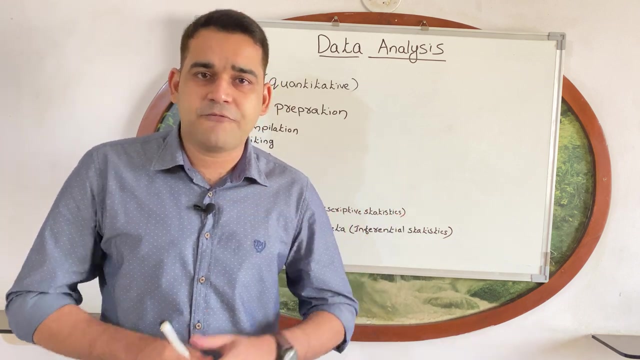 So that questionnaire is used. Using that questionnaire, using that question paper, the teacher is conducting the exam. So teacher is getting the answers. So that answer is used. So teacher is getting the answer, So teacher is getting the answer sheet. is the data. The answer sheet is the data. So to analyze the data after collecting the 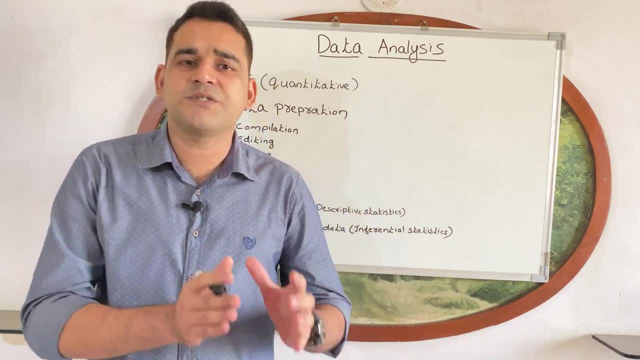 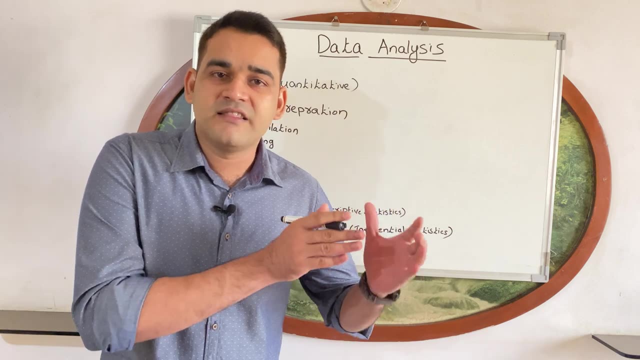 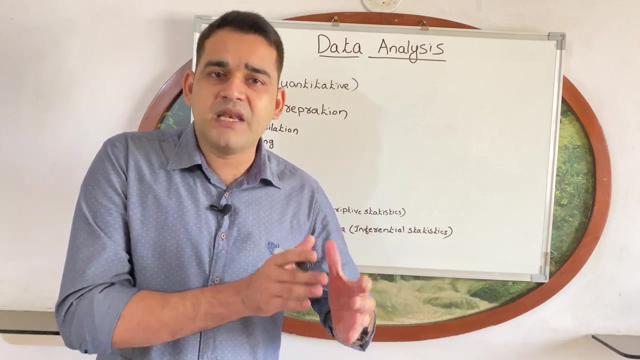 data. in research you have to analyze the data. So what is mean by analysis? Analysis means you are examining that data or you are evaluating that answer sheet. So analysis means evaluating or examining in detail, in depth, In detail you are examining, or in detail you are. 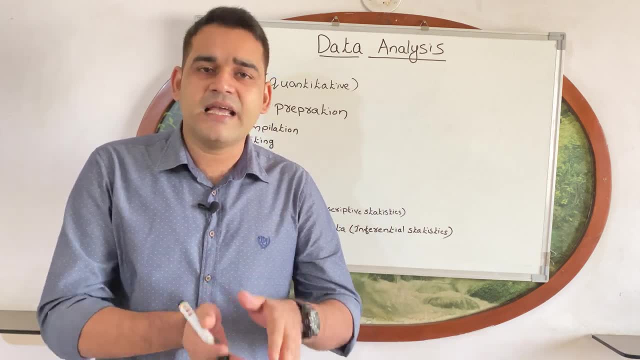 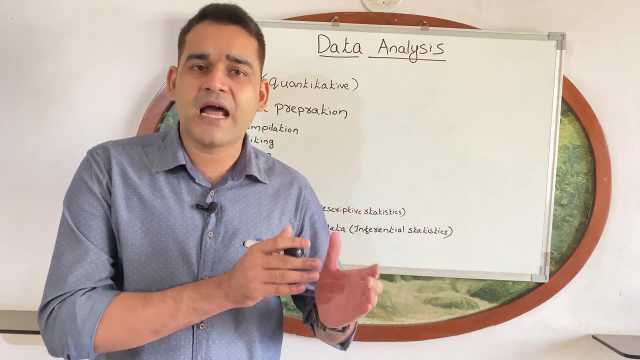 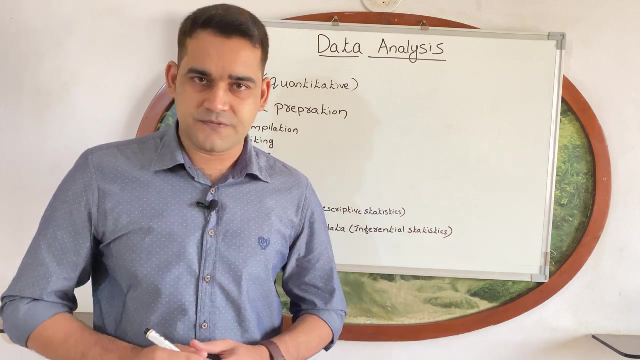 evaluating the data. The data is that answer sheet. I am just giving the example only So we can see the definition of data analysis. So what is mean by data analysis? Data analysis is the process of data analysis is the process of breaking. 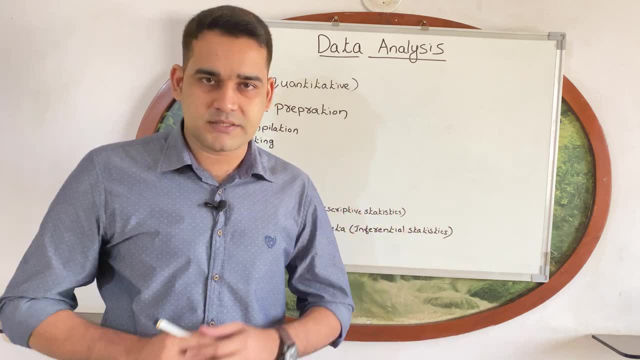 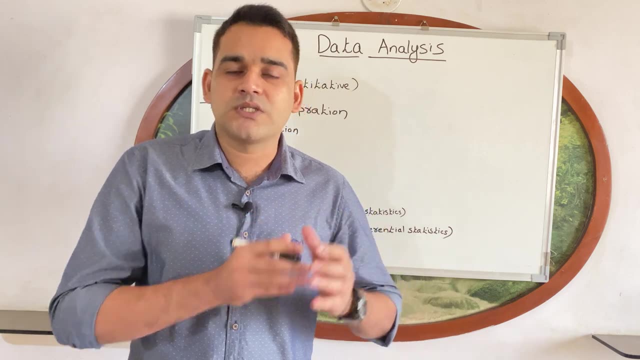 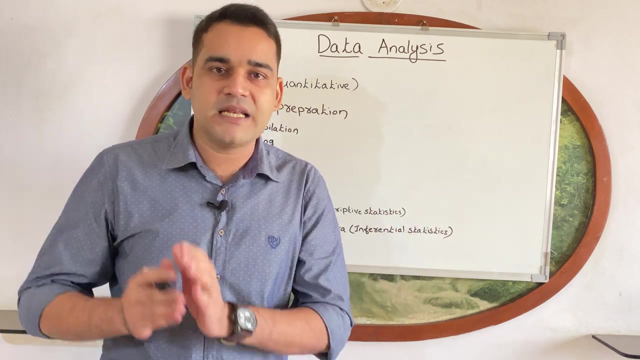 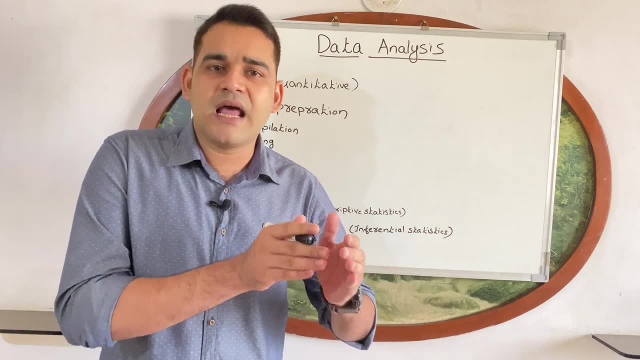 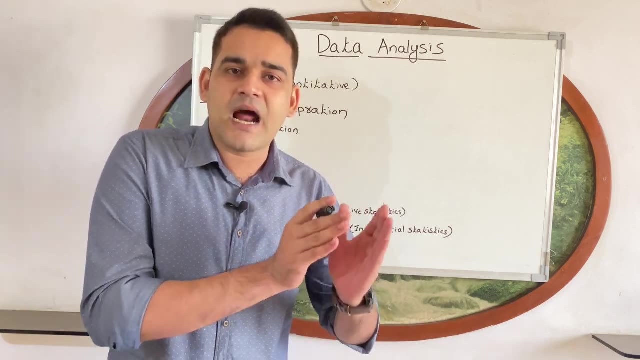 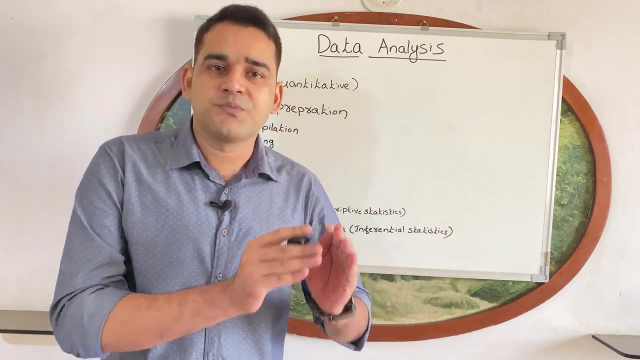 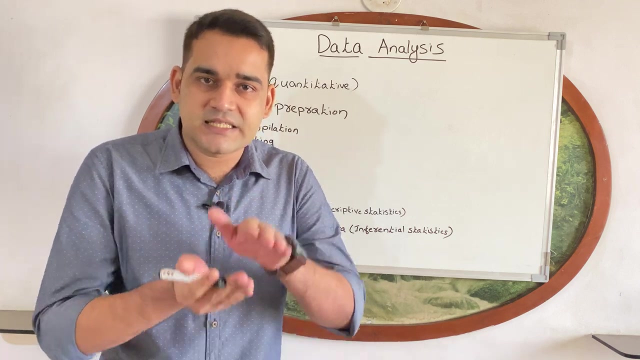 putting marks. So data analysis means you are breaking a big topic to a small one for what? to gain better understanding of it. Data analysis is the process of breaking a complex topic to a smaller part to gain better understanding of it. So all the collected answer sheet, that is the. 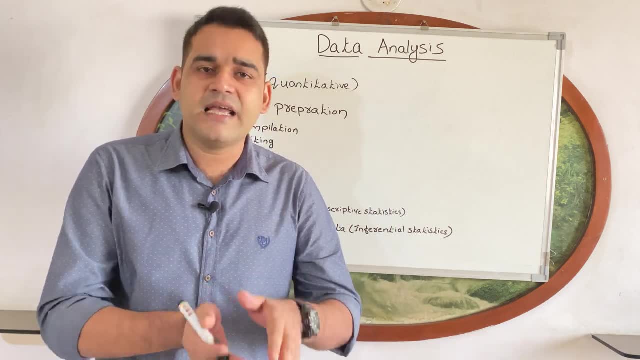 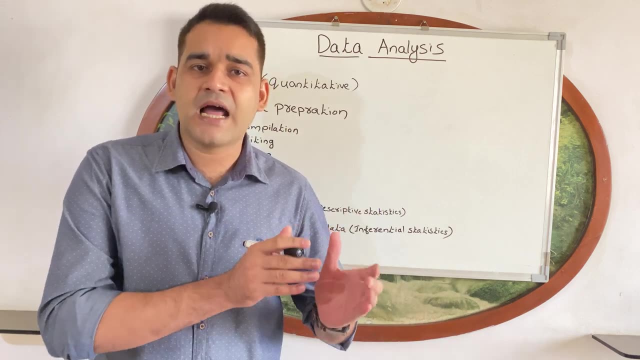 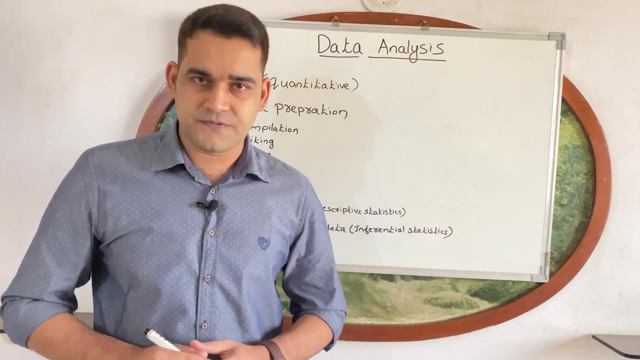 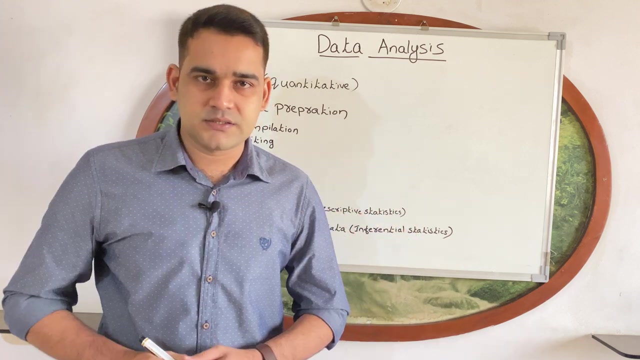 evaluating the data. The data is that answer sheet. I am just giving the example only So we can see the definition of data analysis. So what is mean by data analysis? Data analysis is the process of data analysis, Breaking complex topic to a smaller part to gain better understanding of it. So data analysis is: 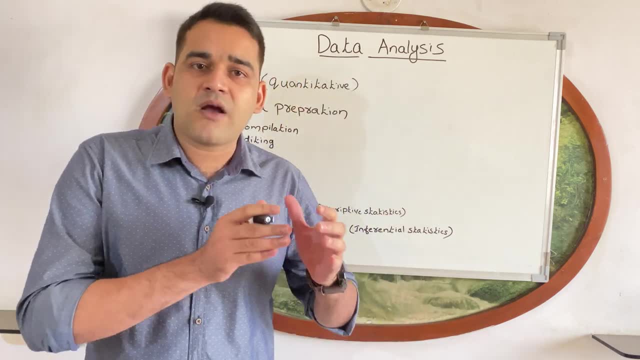 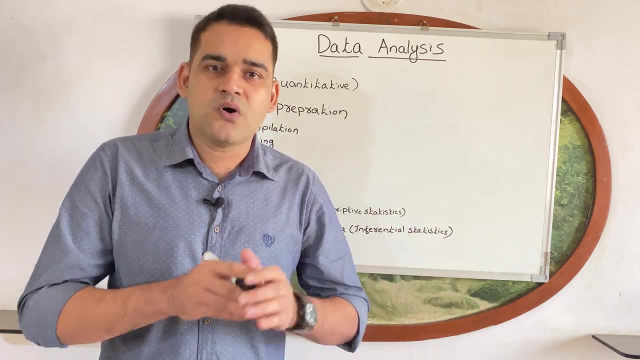 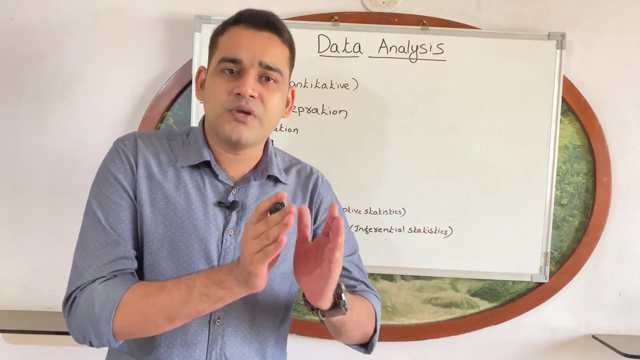 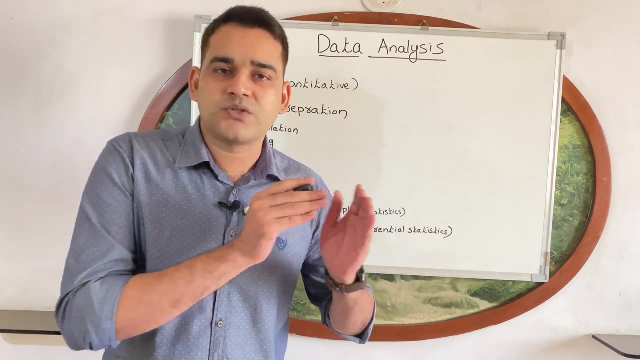 a process of- sorry, breaking a complex topic- that is, that answer sheet- to a smaller part that is putting marks. So data analysis means you are breaking a big topic to a small one For what? To gain better understanding Of it. Data analysis is the process of breaking a complex topic to a smaller part to gain better. 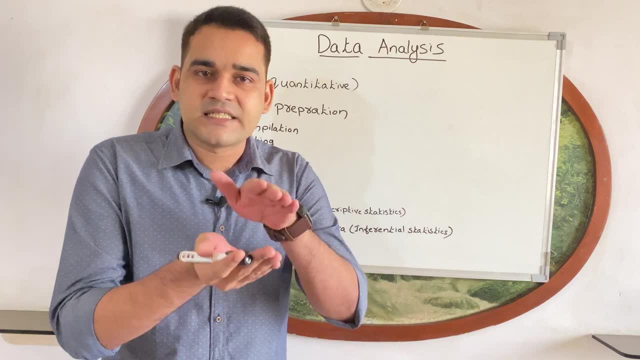 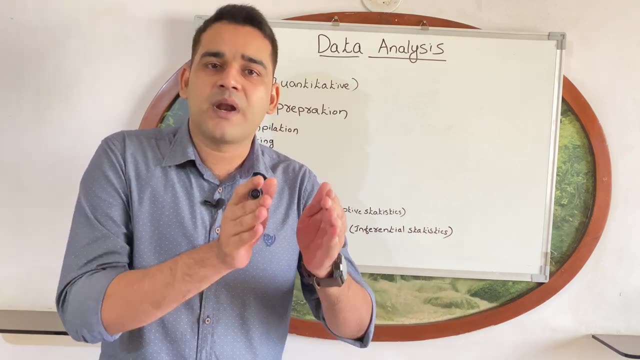 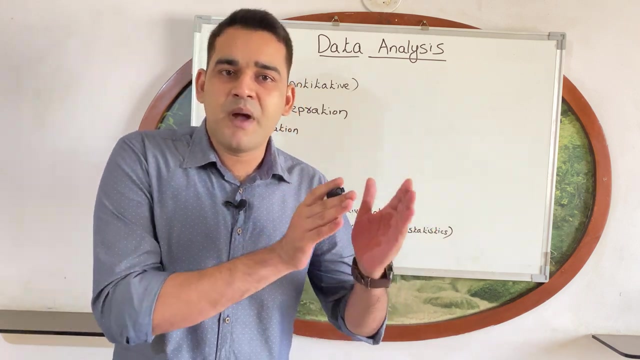 understanding of it. So all the collected answer sheet, that is the complex topic You have break. you have put the mark, So you have break into smaller parts. For what? To gain better understanding. Now the teacher has got a better understanding regarding that answer sheet. 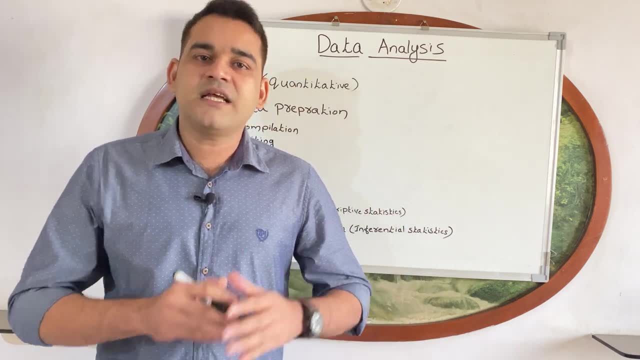 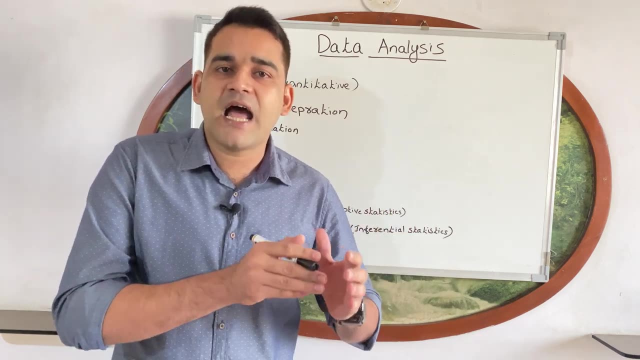 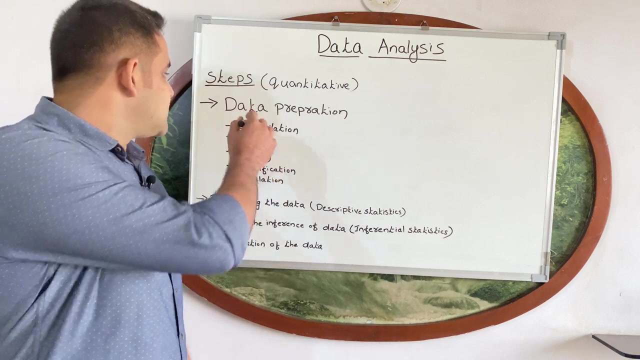 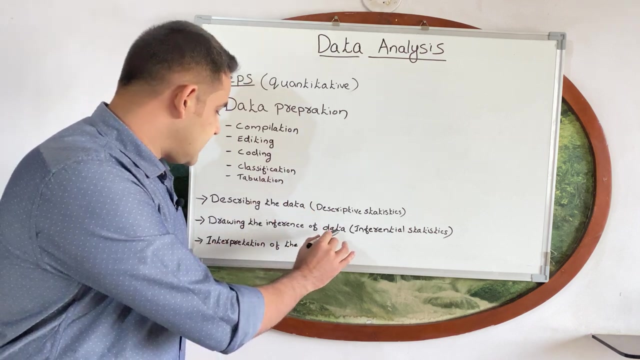 That is data analysis. Next we can see the steps of data analysis in quantitative study, The steps of data analysis in quantitative study. Mainly you can see four steps. First one is data preparation. Second one is describing the data. Third one is drawing the inference of data And fourth one is interpretation of the data. First one is data preparation. Second one is describing the data. Third one is drawing the inference of data And fourth one is interpretation of the data. 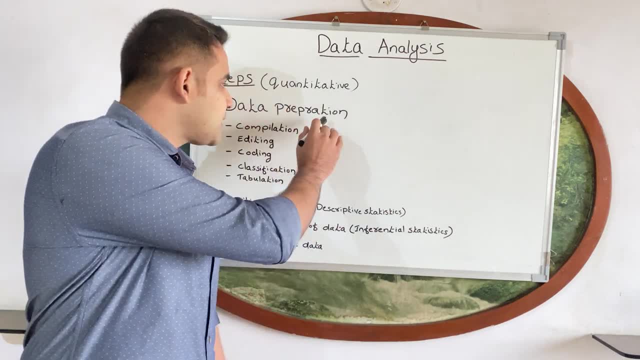 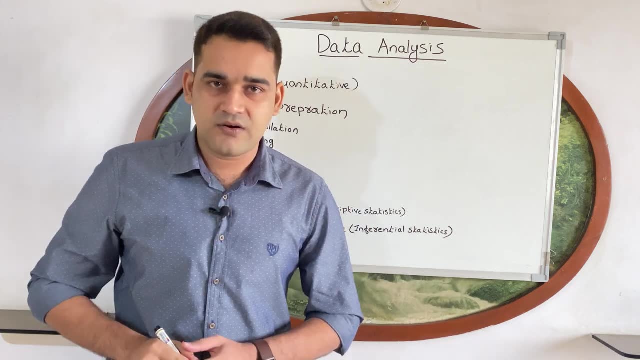 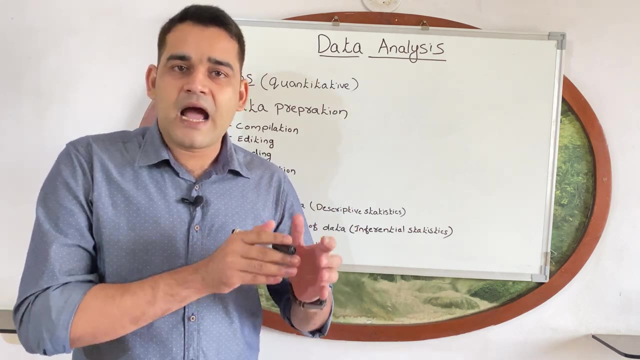 First one is data preparation. Data preparation means you are checking and cleaning the data. You got an idea regarding what is data and what is analysis of data. So the steps of data analysis: first one is data preparation. You are preparing the data In. 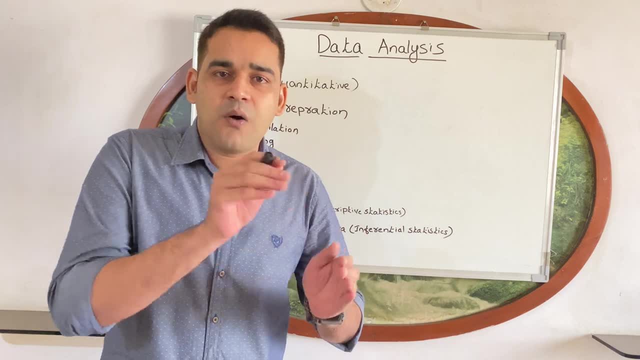 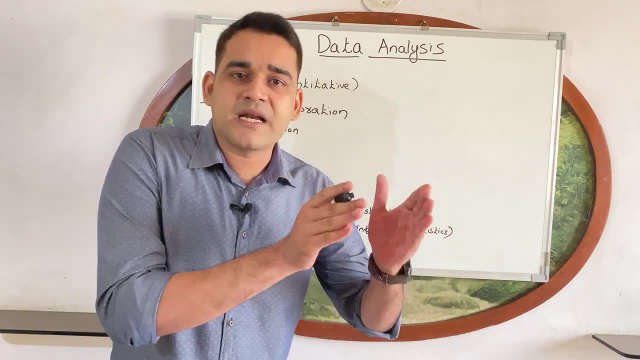 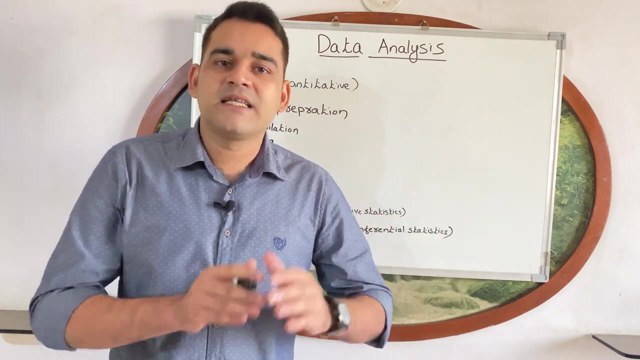 complex topic. You have break. you have put the mark, So you have break into smaller parts. for what? to gain better understanding. Now the teacher has got a better understanding regarding that answer sheet. that is data analysis. Next we can see the steps of data analysis. 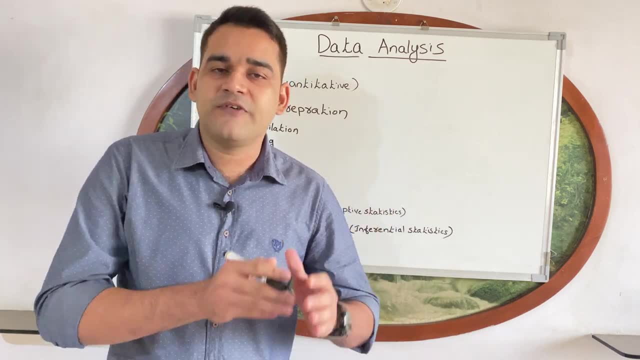 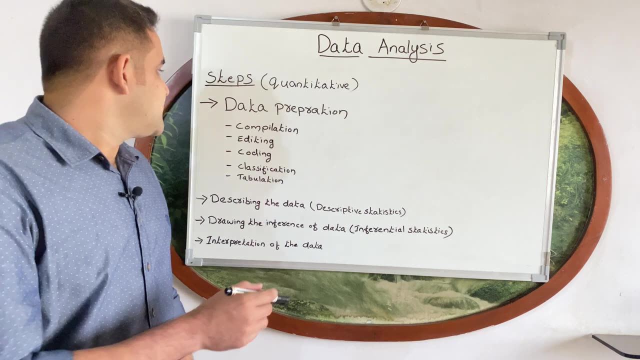 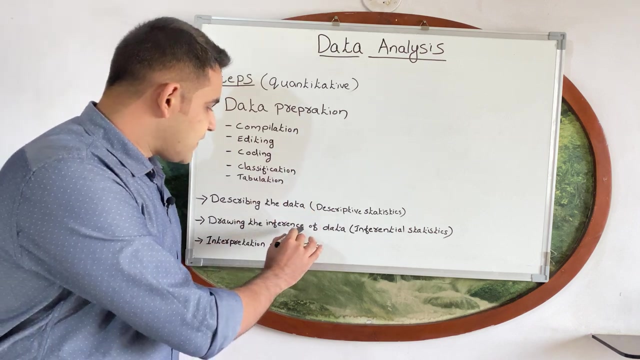 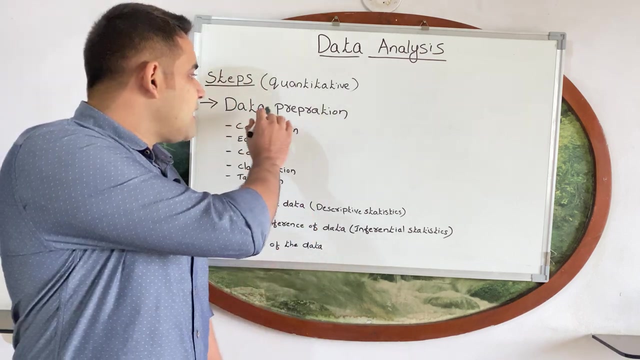 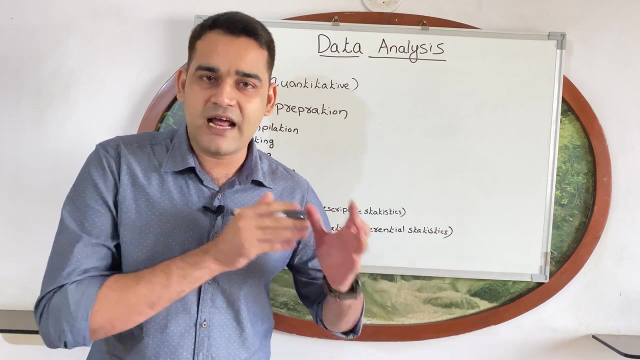 in quantitative study, The steps of data analysis. in quantitative study, mainly you can see four steps. First one is data preparation. Second one is describing the data. Third one is drawing the inference of data and fourth one is interpretation of the data. First one is data preparation. Data preparation means you are checking and cleaning the data. You 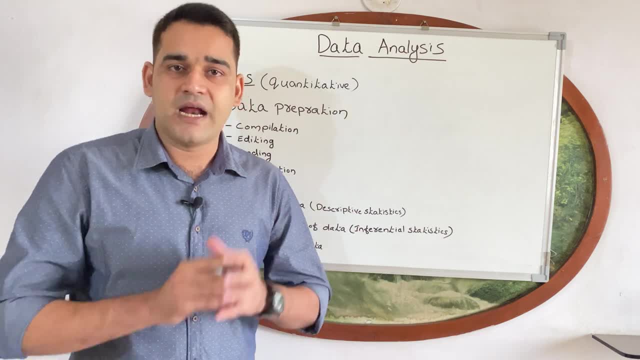 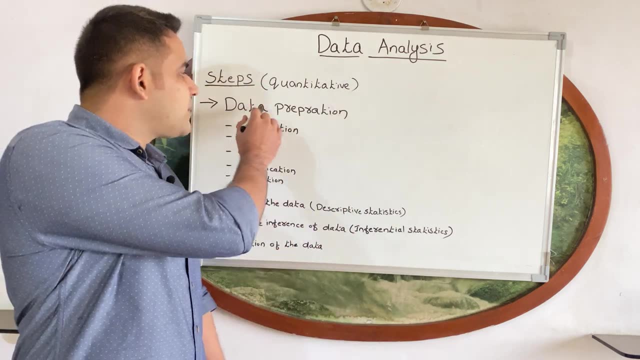 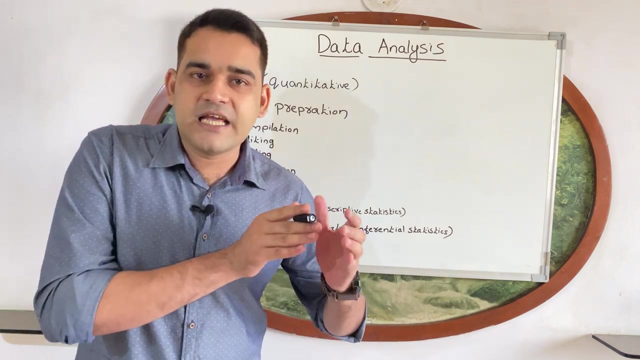 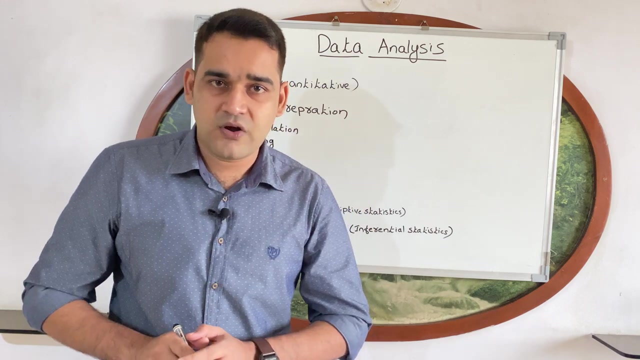 have got an idea regarding what is data and what is analysis of data. So the steps of data analysis: first one is data preparation. You are preparing the data. In preparation of the data, you are checking and cleaning the data. You have to keep it in mind in this step, you are checking as well as you are cleaning the data. okay, it. 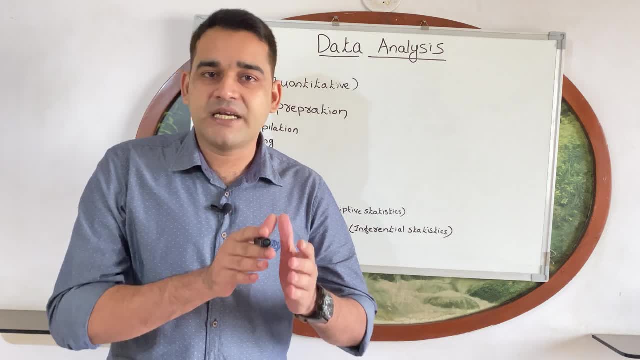 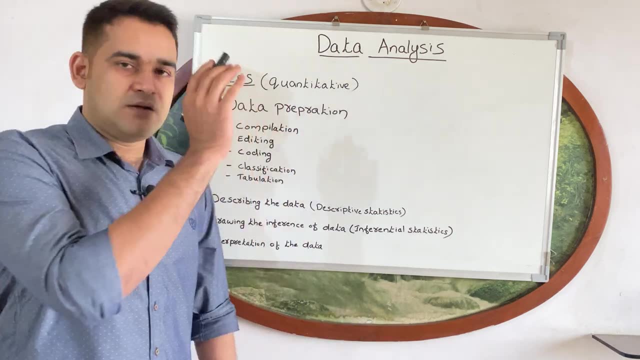 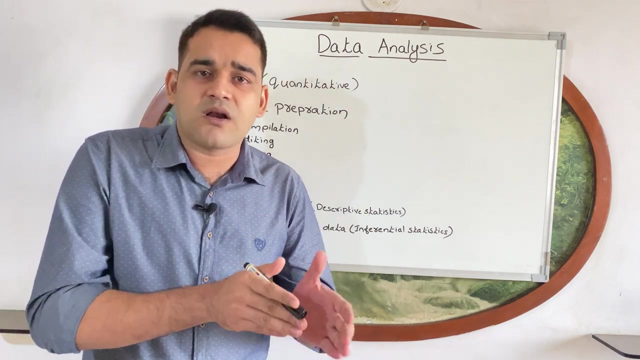 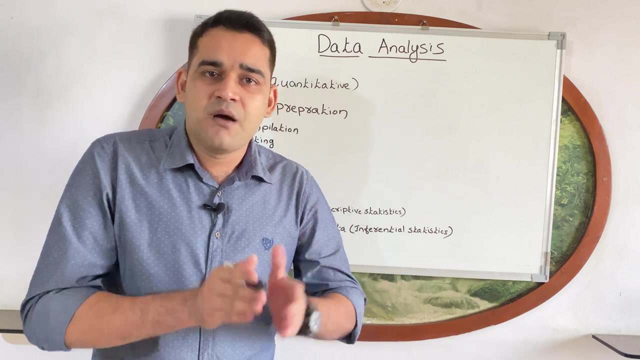 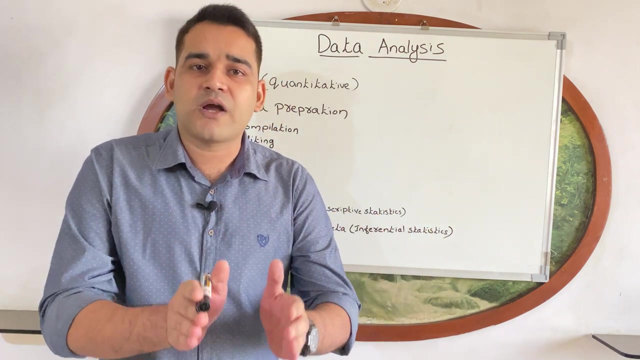 include five sub steps, so you will get a better idea. okay, it include five sub steps. first one is compilation. okay, first one is compilation. so what is mean by compilation? compilation means bringing together all the collected data. okay, so bringing together all the answer sheet collected by the teacher and arranging in a particular order according to the serial number or according 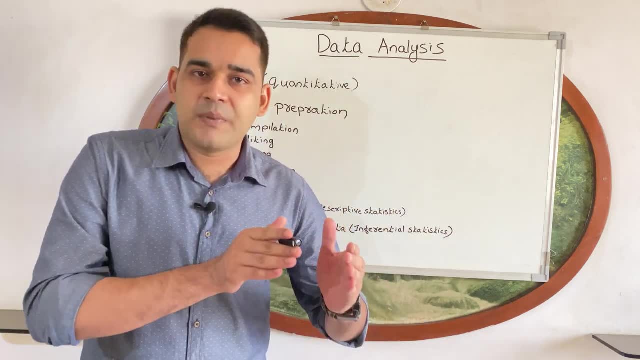 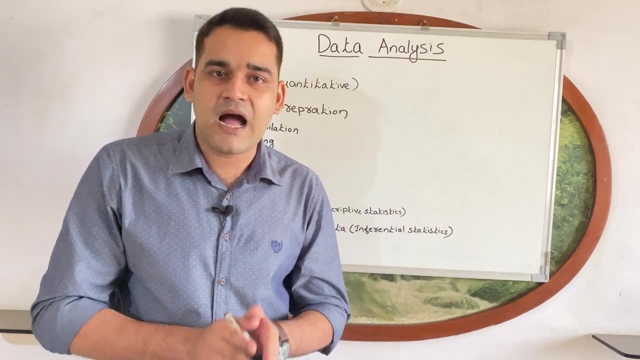 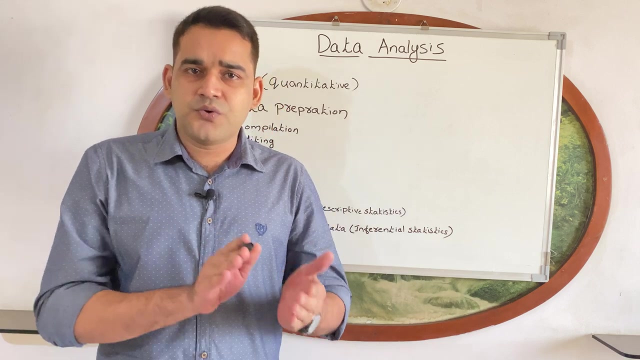 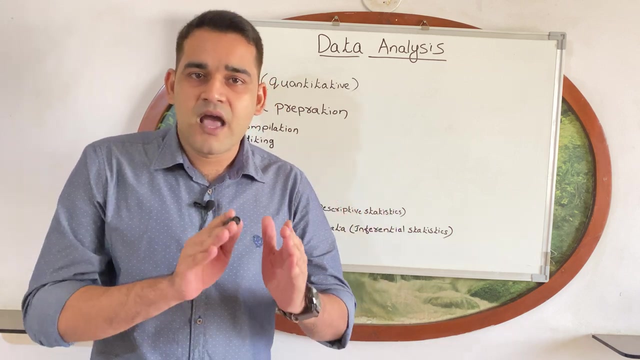 to the roll number of the students. that is compilation. the first step is compilation. that means bringing together all the collected data and arranging in a particular order. that is, your bringing all the collected answer sheet together as well as arranging it in a particular order, that is, according to the serial number or according to the roll number. that is compilation. okay, next step. 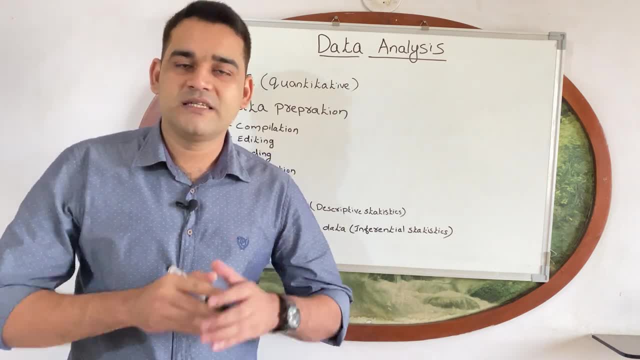 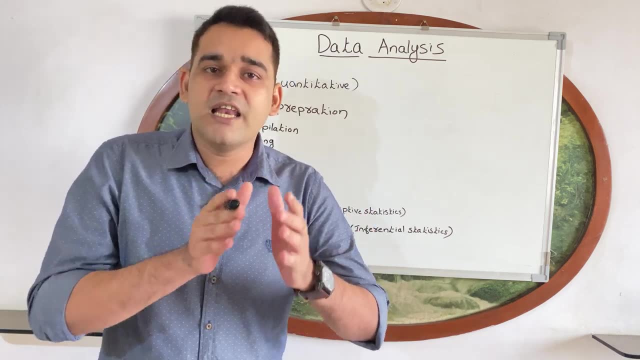 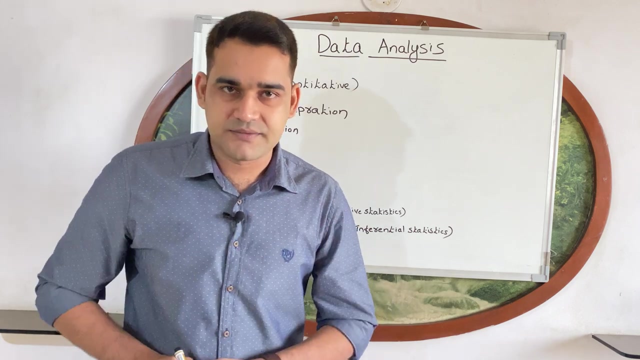 preparation of the data. You are checking and cleaning the data. You are to keep it in mind. In this step, you are checking as well as you are cleaning the data. It includes five sub-steps, So you will get a better idea. It includes five sub-steps. First one is compilation. 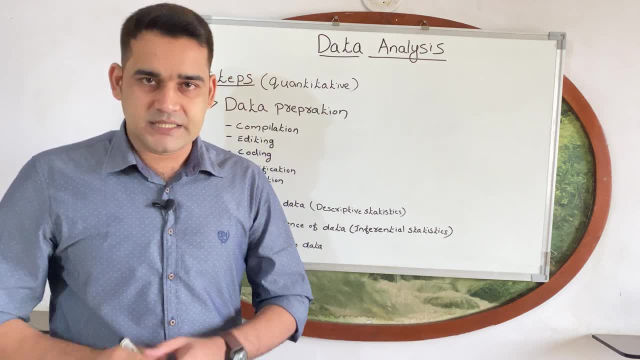 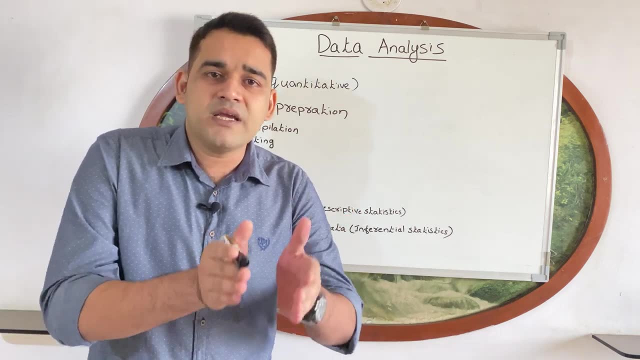 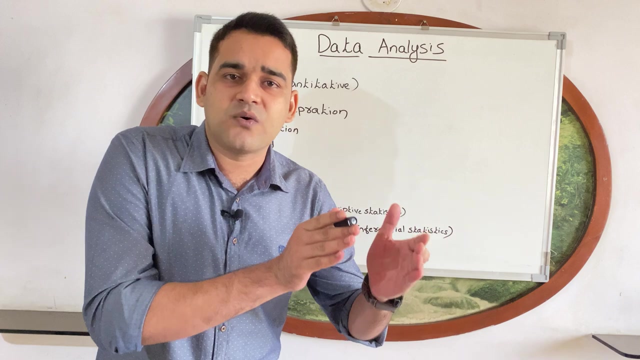 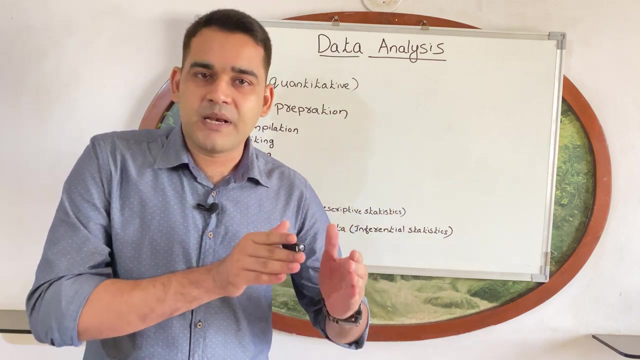 First one is compilation. So what is mean by compilation? Compilation means bringing together all the collected data. So bringing together all the answer sheet collected by the teacher and arranging in a particular order according to the serial number or according to the roll number of the students. That is compilation. The first step is compilation. That means bringing 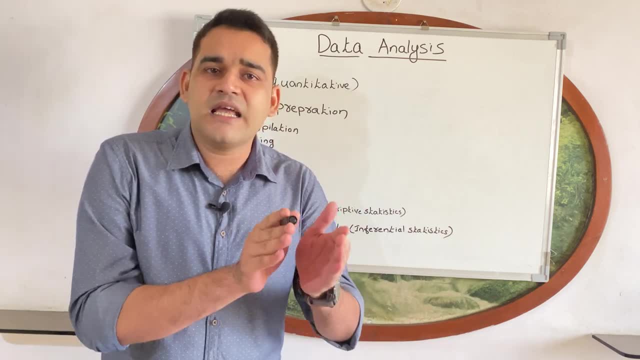 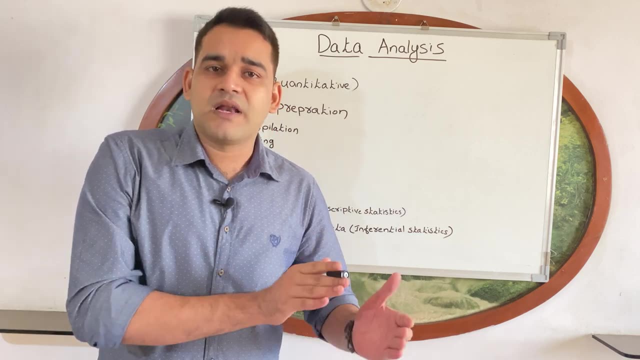 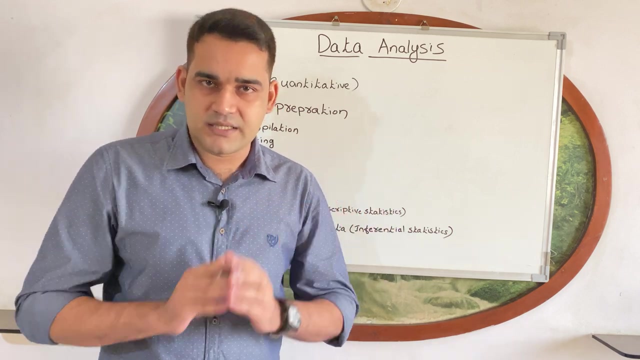 together all the collected data and arranging in a particular order. That is, you are bringing all the collected data, collected answer sheet together as well as arranging it in a particular order, that is, according to the serial number or according to the roll number. that is compilation, ok. 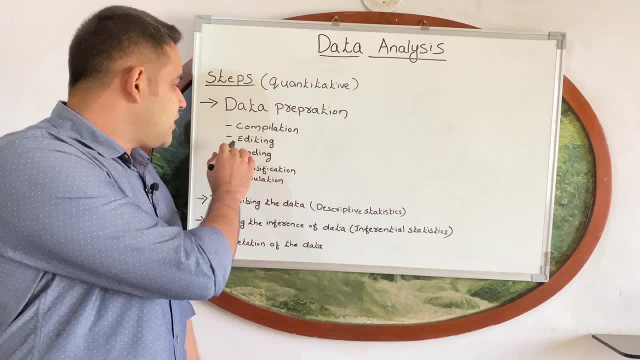 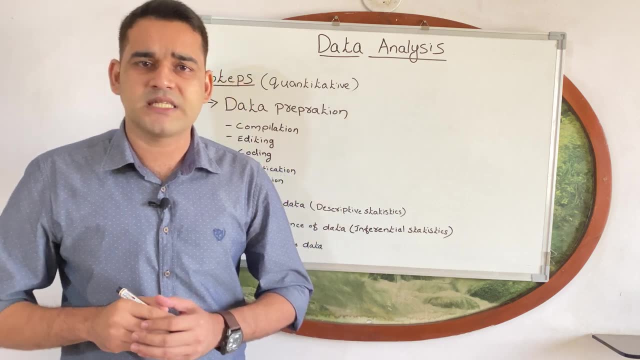 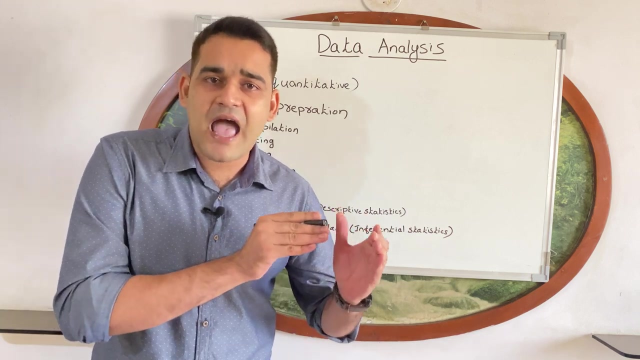 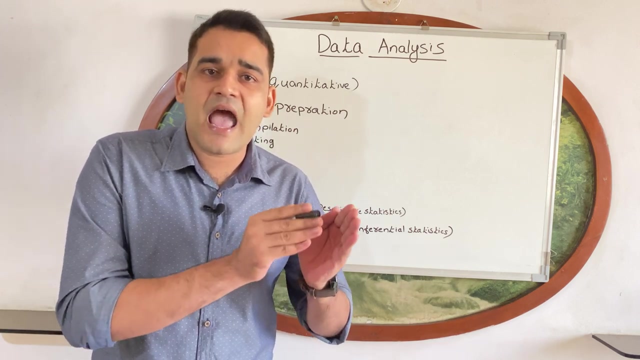 next step is editing. after compilation, you are doing editing. so what is mean by editing? editing means you are checking. it is a process in that you are checking the completeness, utility as well as the accuracy of the answer. ok, the researcher is checking regarding the completeness and the accuracy of the answer. that means all the answers, all the questions. 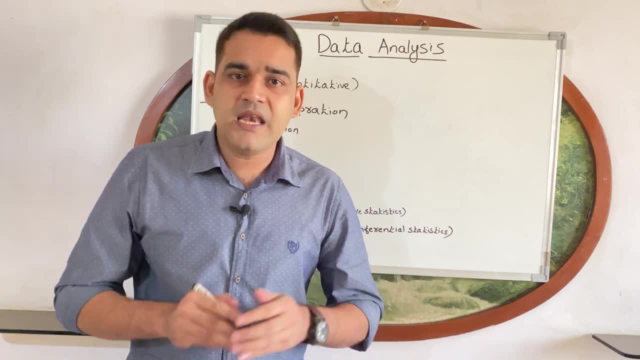 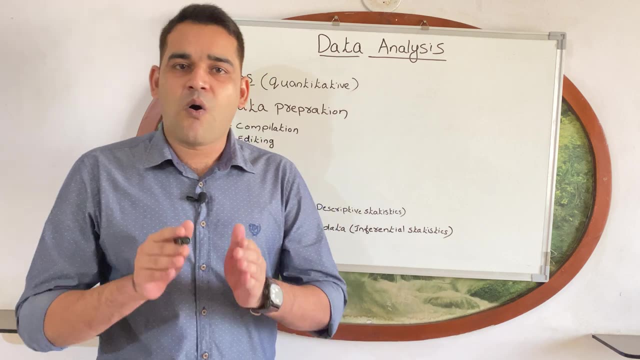 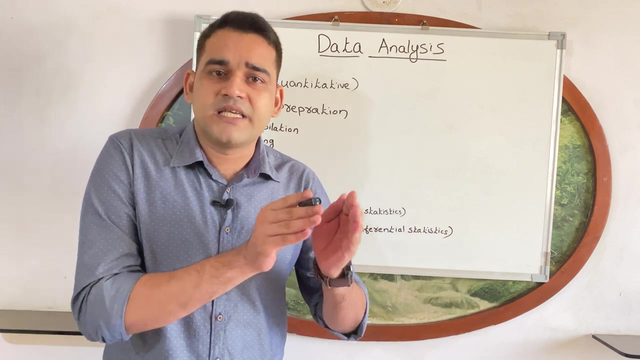 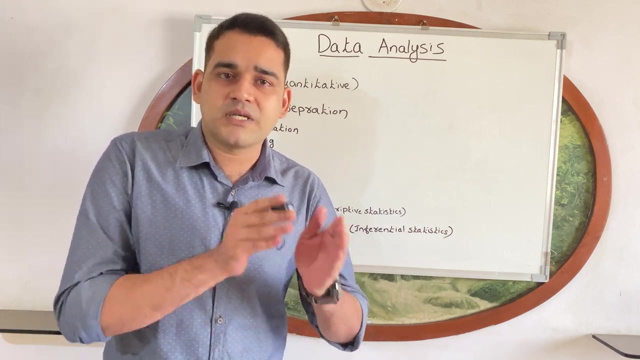 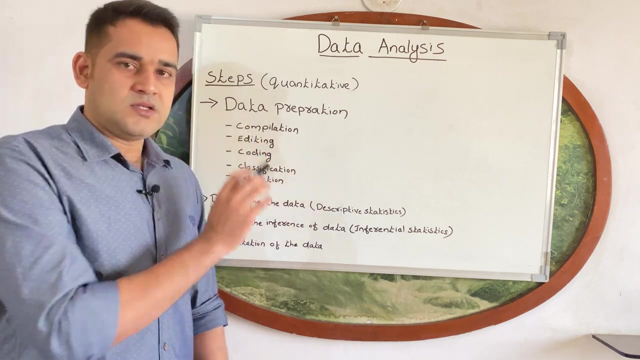 are answered properly or not. any questions has skipped or not is checked. in this step in editing, the researcher is checking all the questions in the question paper is answered or not. is there any question is skipped? ok, so that is editing. checking the completeness as well as the accuracy of the answer is called editing. ok, next one is coding. so what is mean? 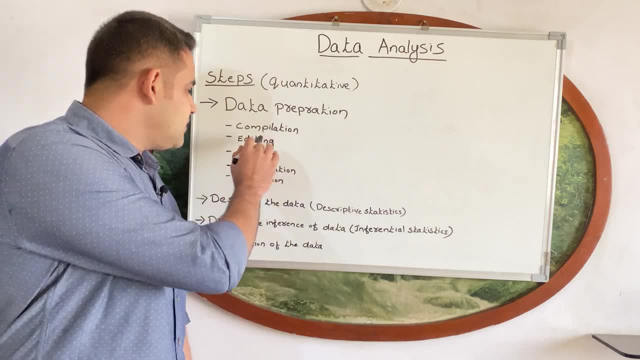 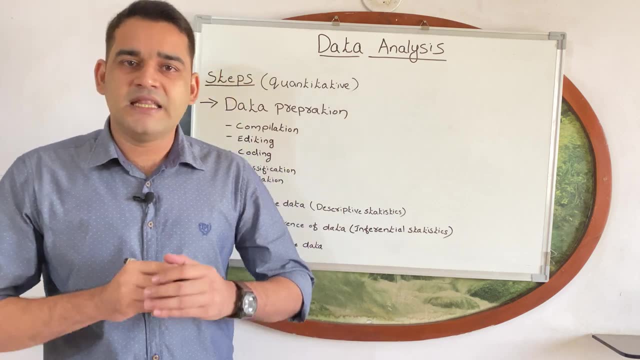 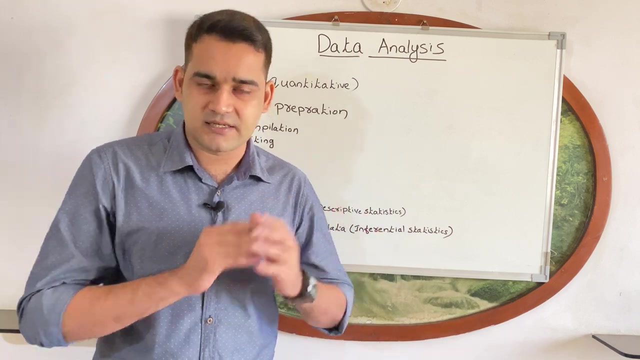 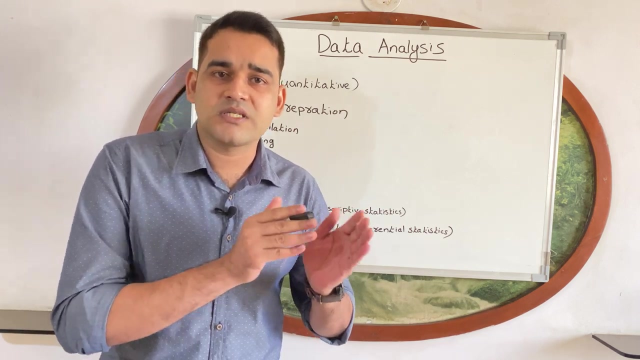 is editing. after compilation, you are doing editing. so what is mean by editing? editing means you are checking. it is a process in that you are checking the completeness, utility as well as the accuracy of the answer. okay, the researcher is checking regarding the completeness and the accuracy of the answer. 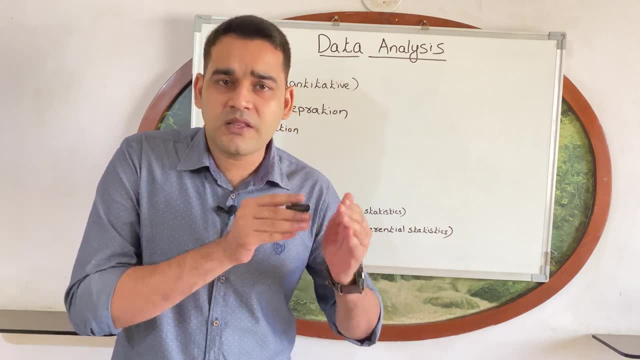 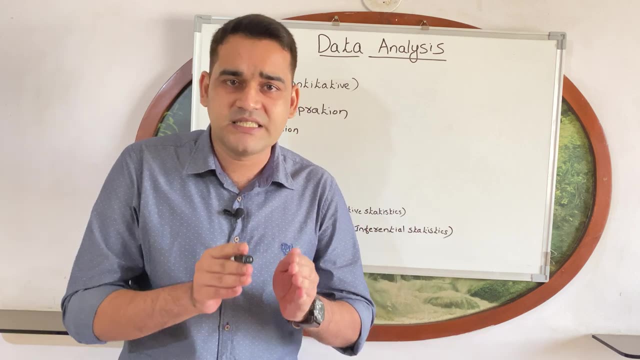 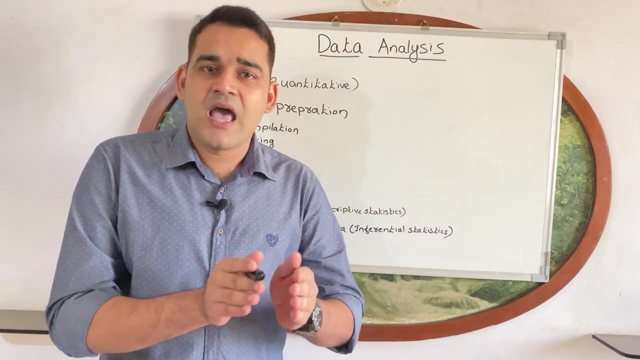 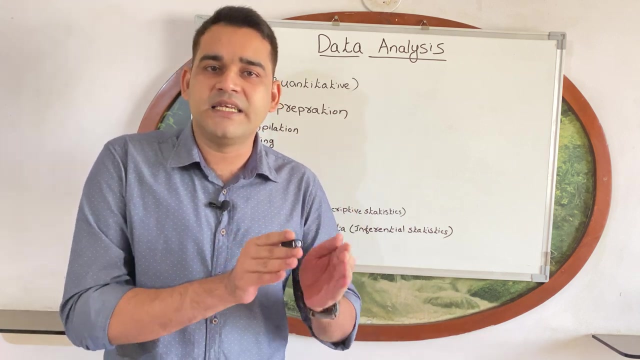 that means all the answers, all the questions are answered properly or not. any questions has skipped or not is checked in this step in editing. the researcher is checking all the questions in the question paper is answered or not. is there any question is skipped? okay, so that is editing. 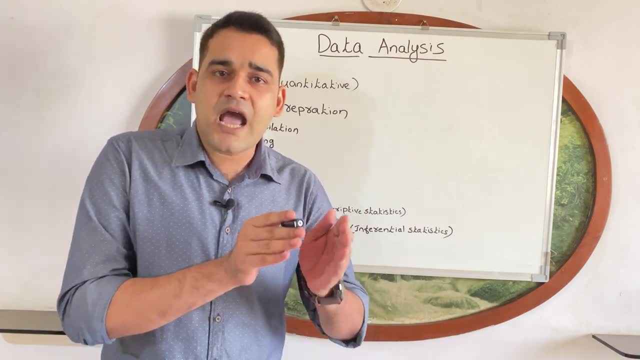 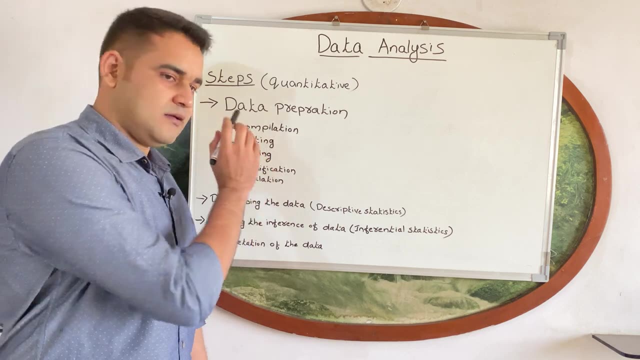 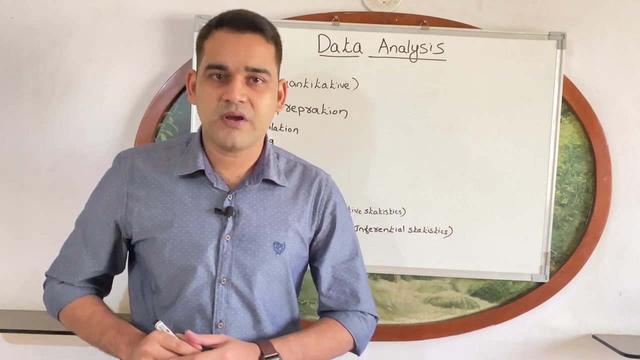 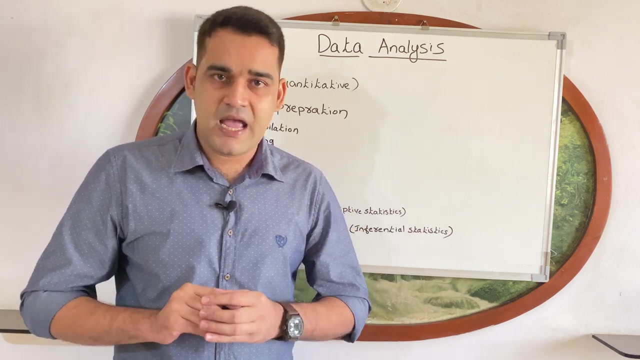 checking the completeness as well as the accuracy of the answer is called editing, okay, next one is coding. so what is mean by coding? coding means transforming the statement into a symbol. okay, transforming the statement into a symbol, that means suppose a statement and making that statement a symbol. it may be in number or it may be in. 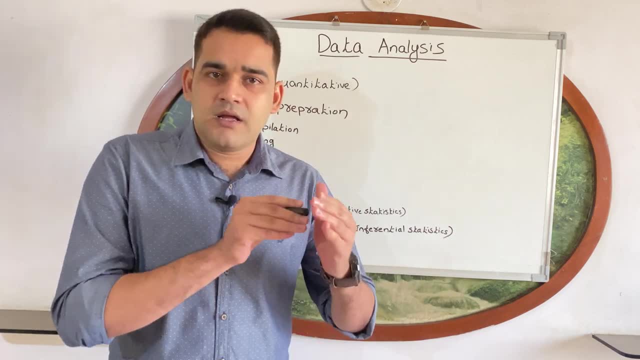 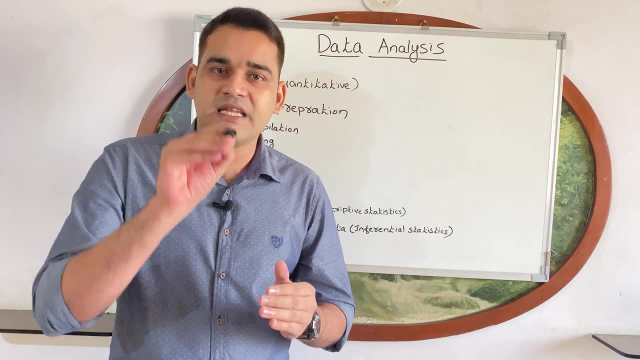 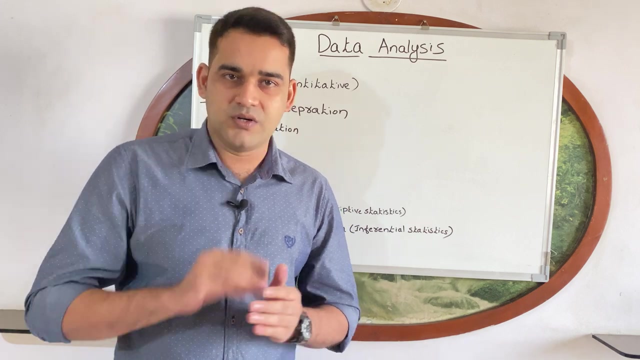 alphabet. okay, suppose, for example, in your study, in your data, for male, okay, you are giving a code that is one. okay, for male you are giving a code one. so you are using a numerical code. for male you are giving a code that is one and for female you are giving a code number twoDo you have any idea really? ways of luminance. 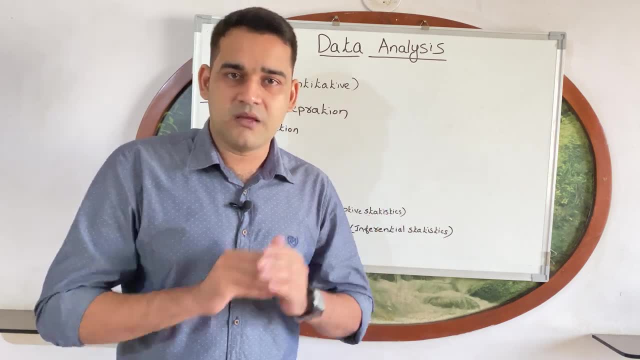 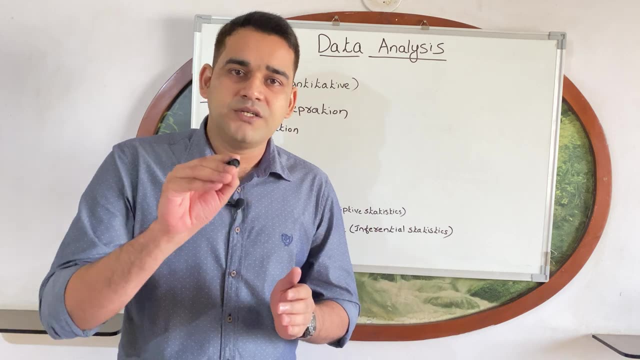 means equal or equal release. it is basically anything that is not consuming law. more i will see. and you are giving the code to. that is coding: transforming the statement to a symbol. The symbol may be alphabet or number. It may be 1,, 2, like that in number, or in A, B, C, like that in. 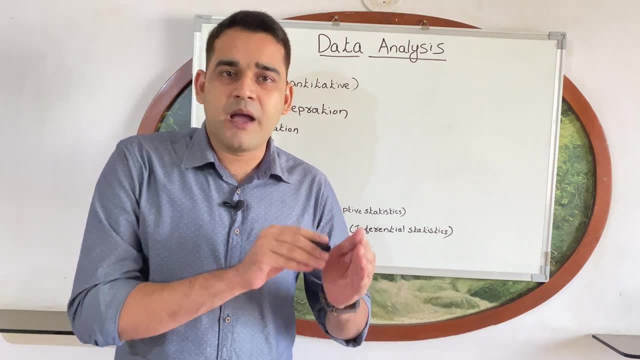 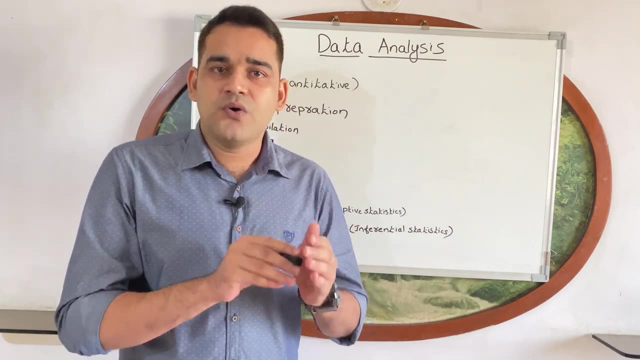 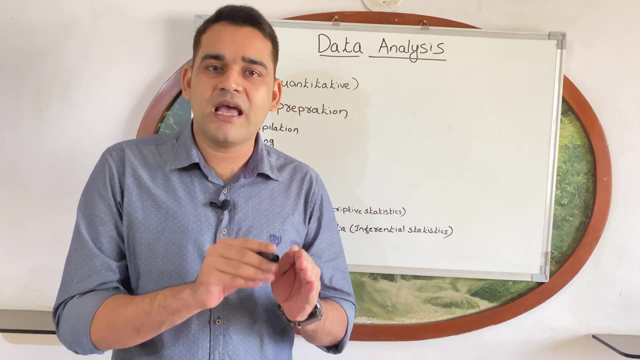 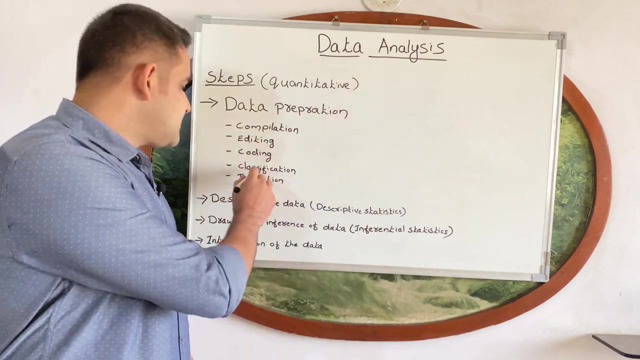 alphabet. also Always keep it in mind: for one character only you should give one code. If you use number 1 for mail, so you cannot use that number 1 to any other statements. So you are making a symbol for a statement. that is coding. Next one is classification. After coding: 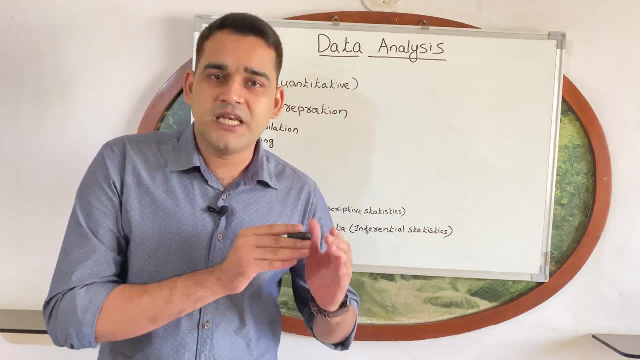 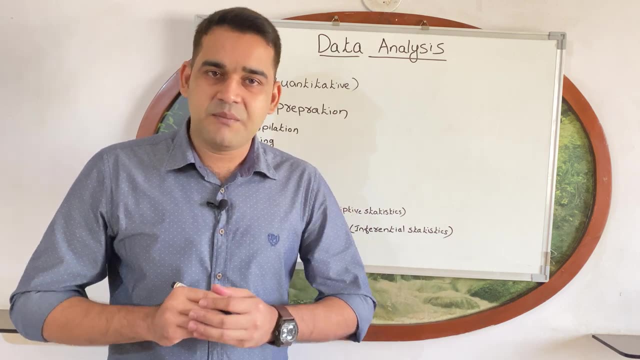 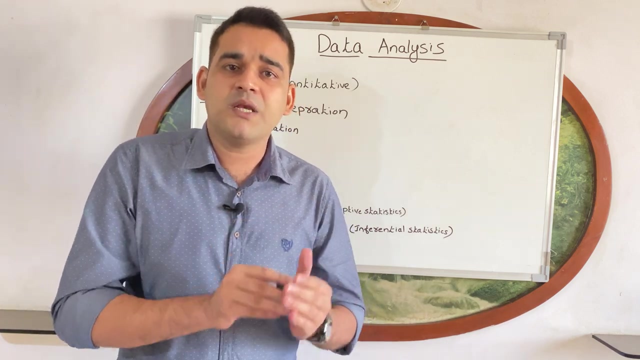 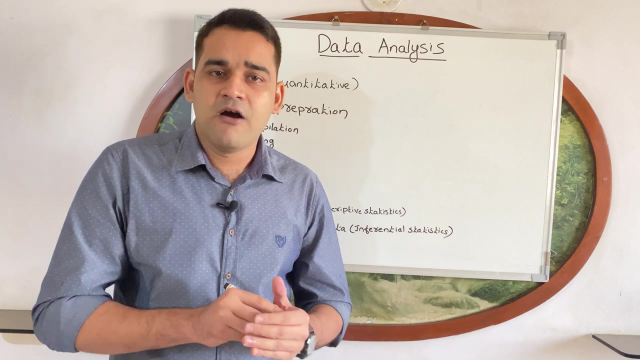 by coding. coding means transforming the statement into a symbol. ok, transforming the statement into a symbol, that means suppose a statement and making that statement to a symbol. it may be in number or it may be in alphabet. ok, suppose, for example, in your study, in your data for male: ok, you are giving. 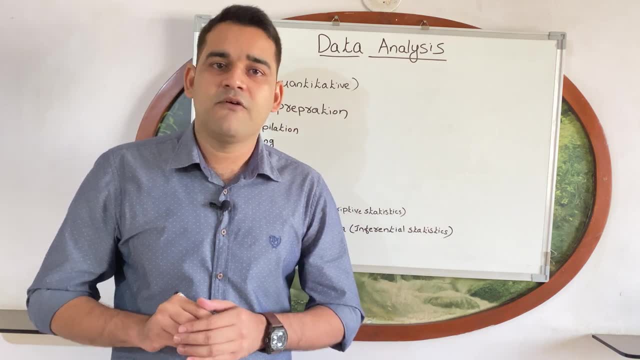 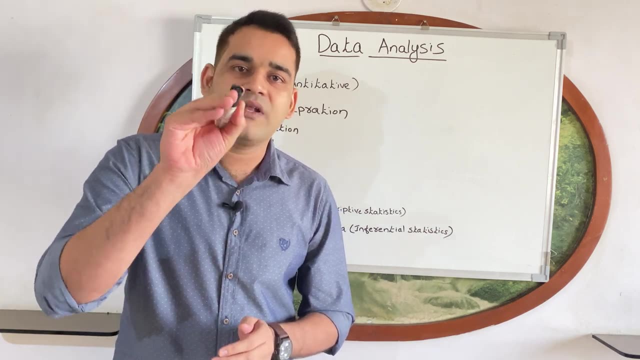 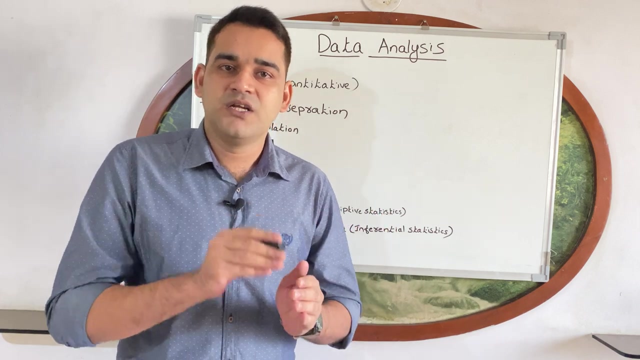 a code that is one. ok, for male, you are giving a code one. so you are using a numerical code. for male, you are giving a code that is one, and for female, you are giving the code two. that is coding, transforming the statement to a symbol. the symbol may be alphabet or. 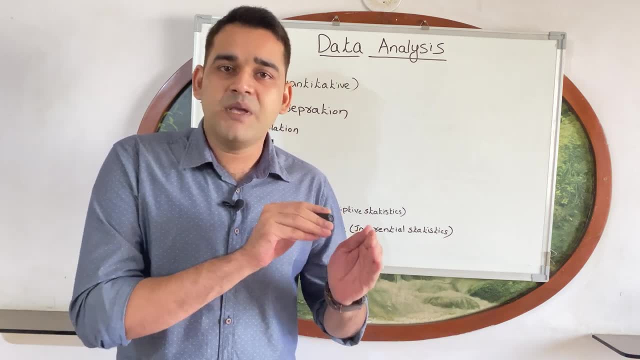 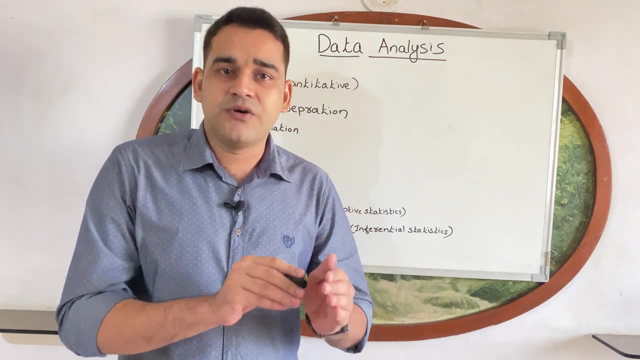 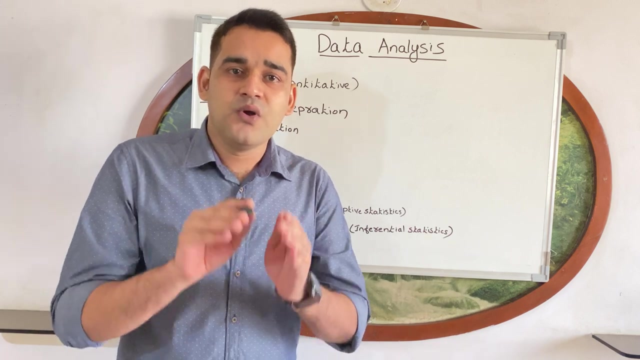 number. it may be one, two, like that in number, or in a, b, c, like that in alphabet. also, ok, always keep it in mind. for one character only you should give one code if you use number one for male, so you cannot use that number one to any other statements. ok, so you are making. 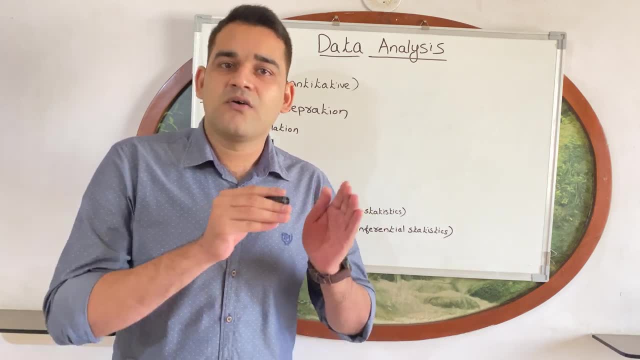 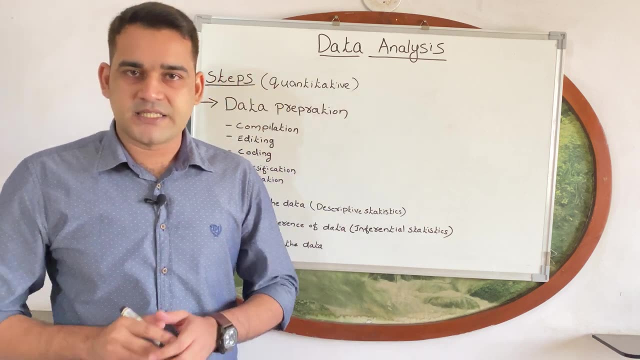 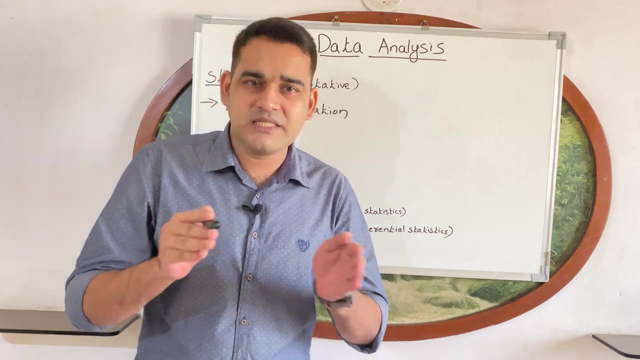 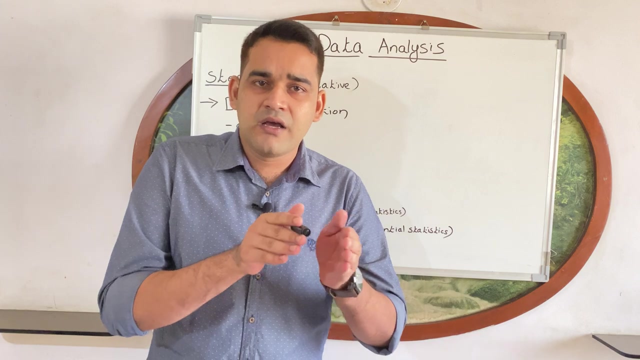 a symbol for a code. ok, ok, a statement. That is coding. What is Next one is classification After coding. classification After coding. you have to classify the data. In some research, there will be so much data will be there, So much data will be there. So it should be classified according to the groups, as 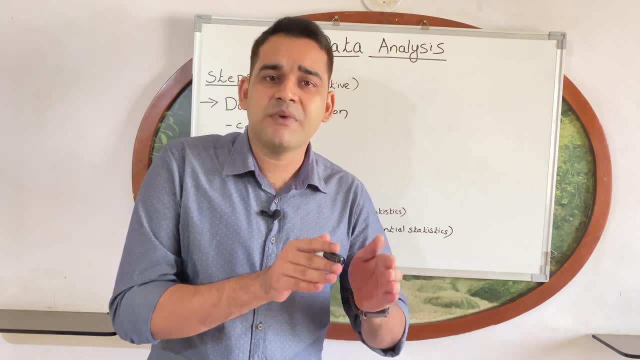 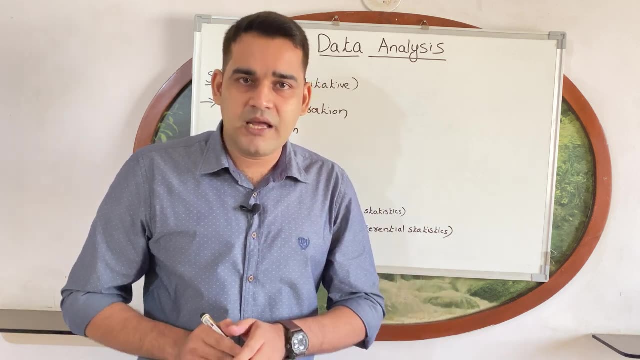 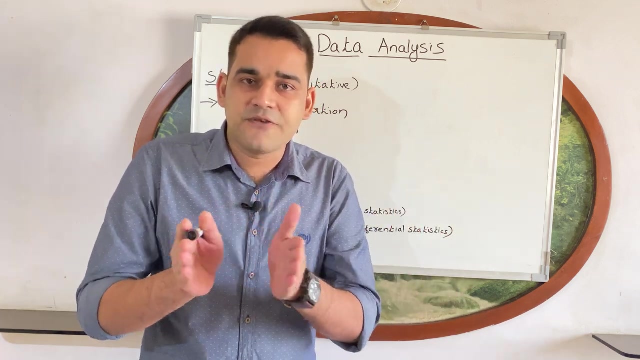 well as according to the particular classes having same characters, For example, male as well as female. you are classifying that data According to the group or according to the class level. you are arranging the data. You are classifying the data: Those having common characters. 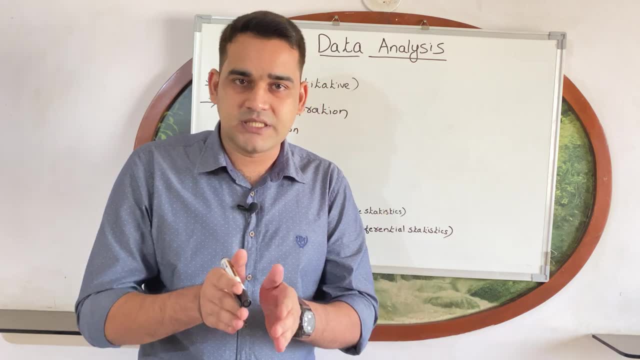 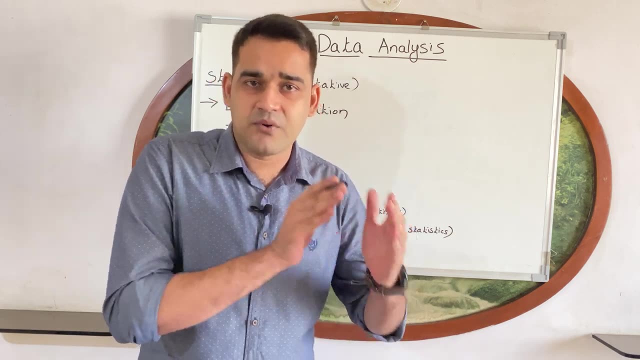 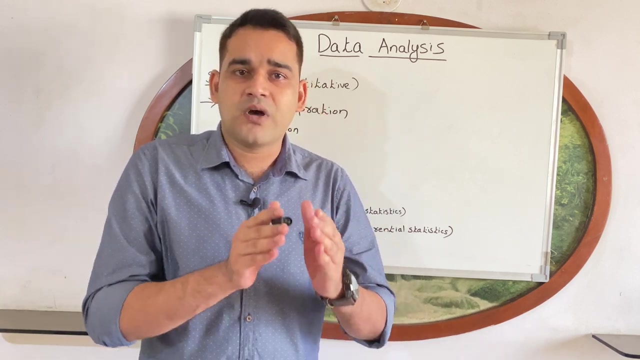 having particular mark range from 50 to 60, you are classifying that data in an order Like that for male and female. I am just giving the example only. So classification means you are classifying the data in particular classes or in particular group: those who are having common characters. 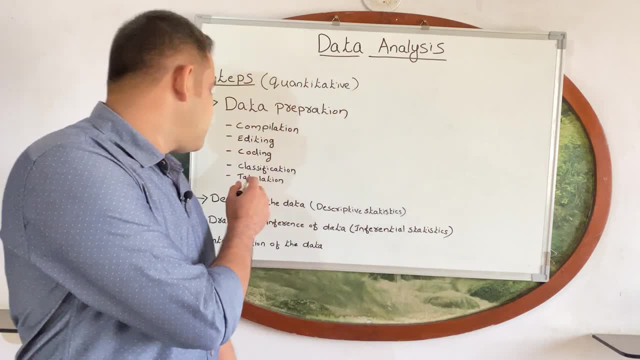 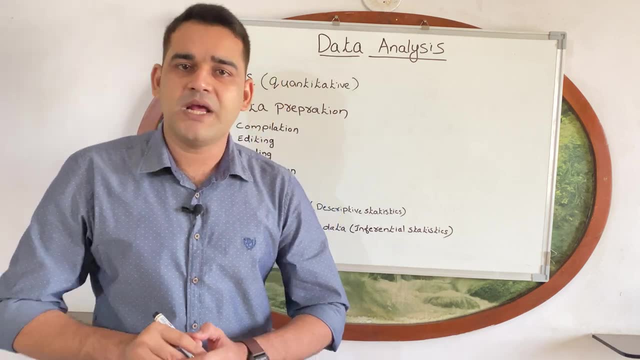 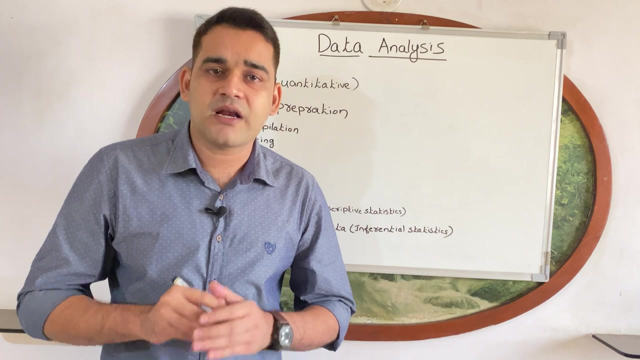 That is classification. Next one is tabulation. After classification, it is tabulation. So what is mean by tabulation? Tabulation means recording the classified data in mathematical terms. You are recording the classified data in mathematical terms. You are recording the. 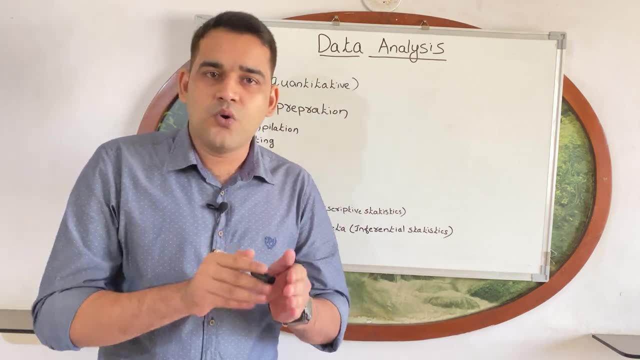 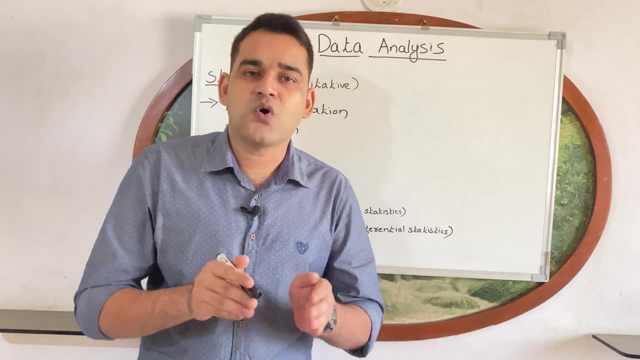 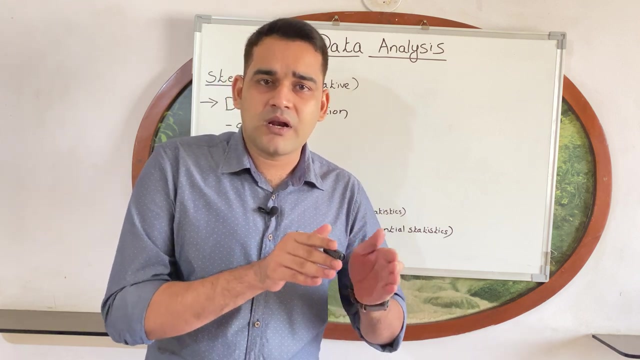 classification. After coding, you have to classify the data. In some research, there will be so much data will be there. So much data will be there. So it should be classified according to the groups as well as according to the particular classes having same characters, For example, male as well as female. 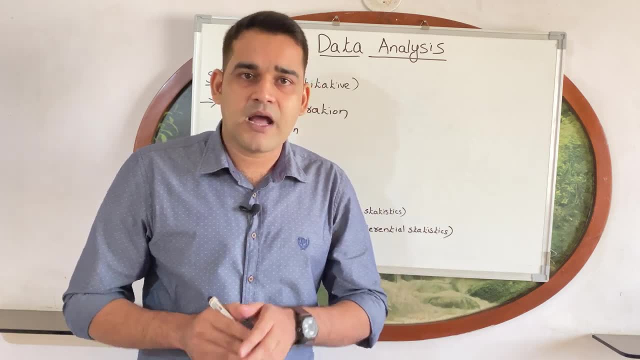 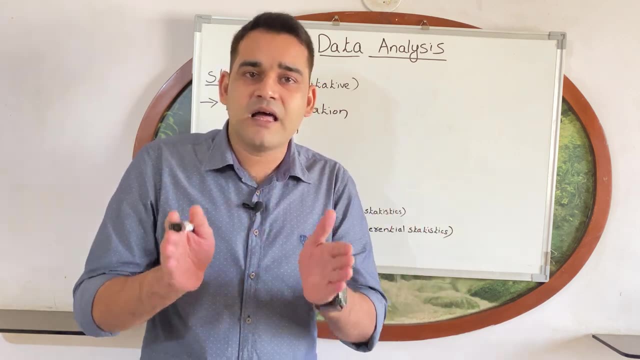 you are classifying that data According to the group or according to the class level. you are arranging the data, You are classifying the data. those having common characters, having particular mark, range from 15 to 20.. So you are classifying the data, So you are classifying the data. So 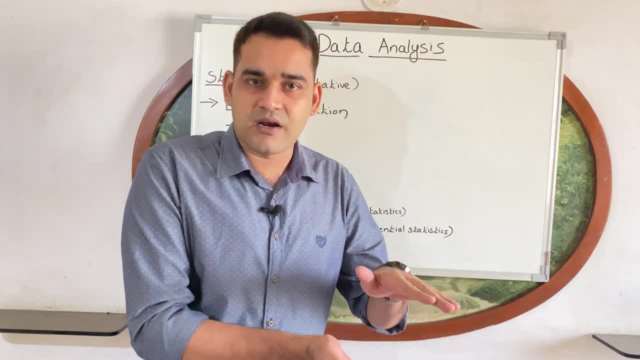 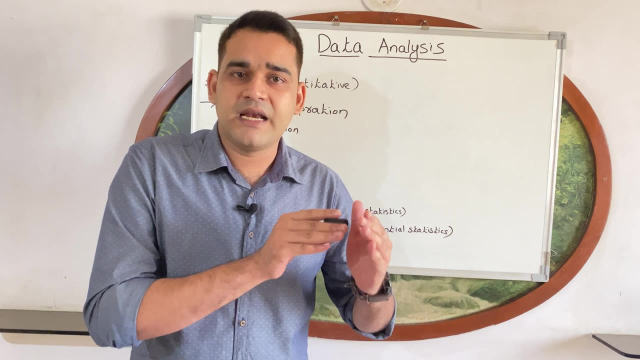 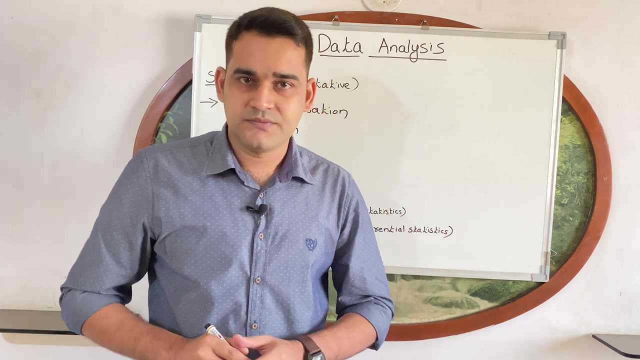 B to 60, you are classifying that data in an order Like that for male and female. I am just giving the example only. So classification means you are classifying the data in particular classes or in particular group- those who are having common characters. That is classification. 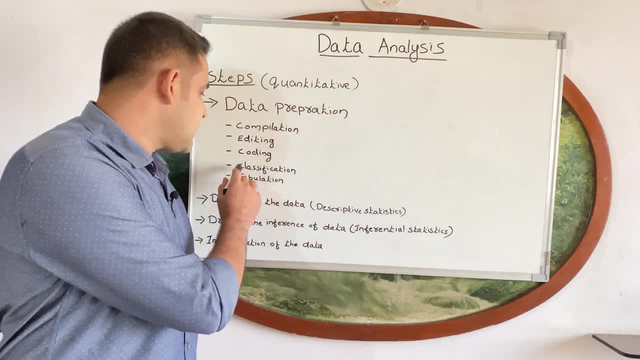 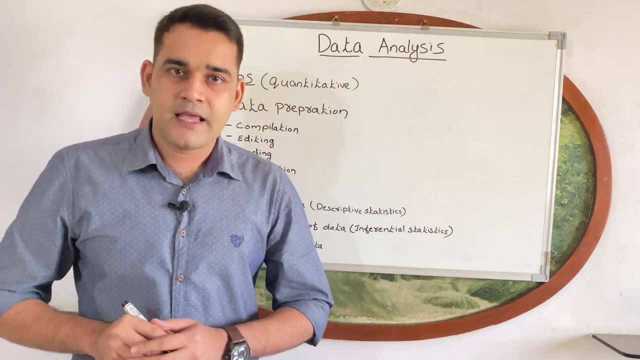 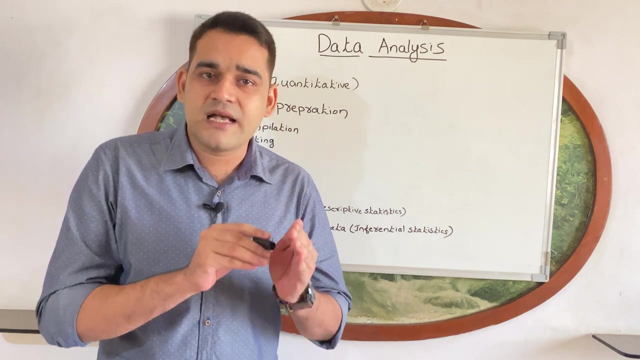 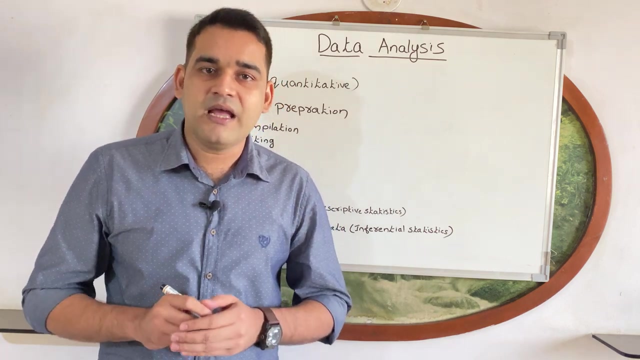 Next one is tabulation. After classification, it is tabulation. So what is mean by tabulation? Tabulation means recording the classified data in mathematical terms. You are recording the classified data in mathematical terms. In simple, you can call it as tables. In simple, you can call it as tables. 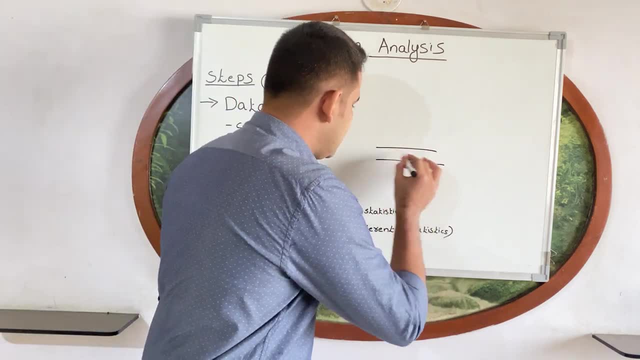 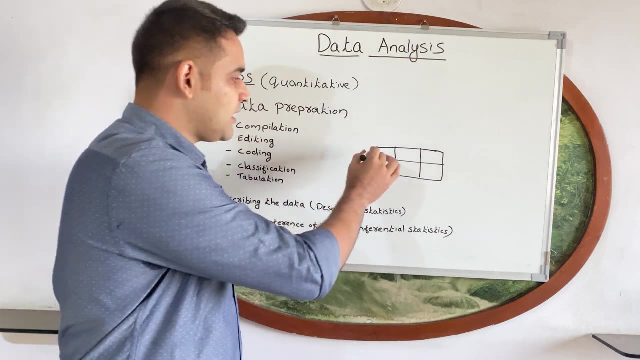 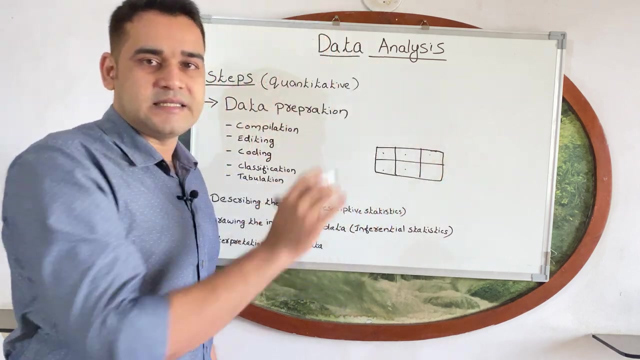 That is in rows as well as in columns. you can make, For example- I am just giving This is tabulation Here you can write male, female, their number of male and as well as number of females, their marks, Like that tables you are making. 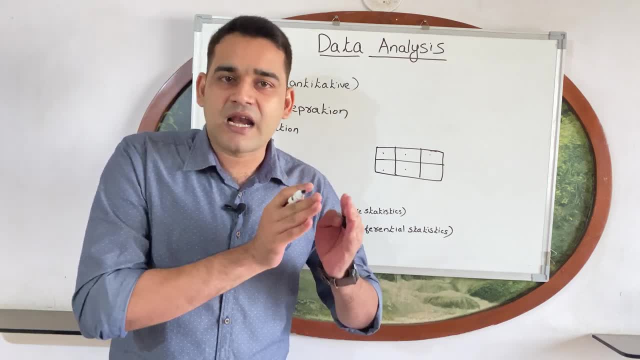 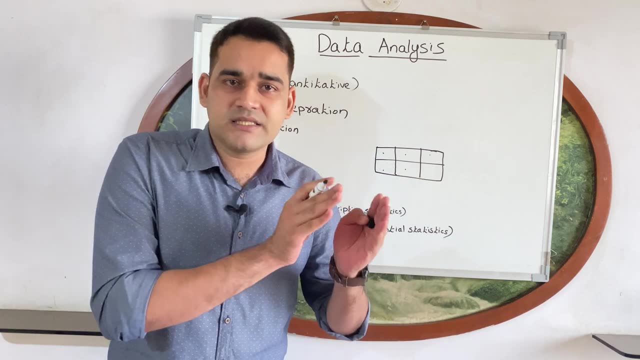 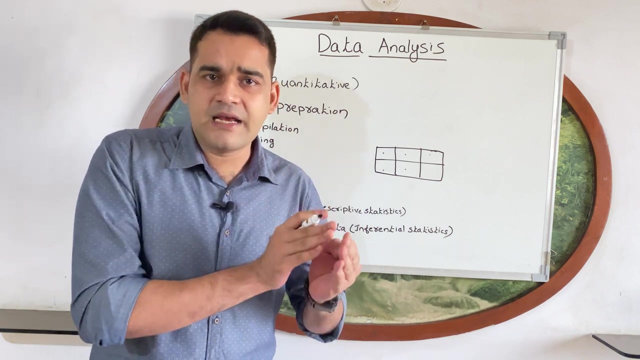 That is tabulation. Tabulation means recording the classified data in mathematical terms. That is, using tables, That is, rows as well as in columns, In rows as well as in columns. you are writing regarding the classified data: How many males are there? How many females are there? 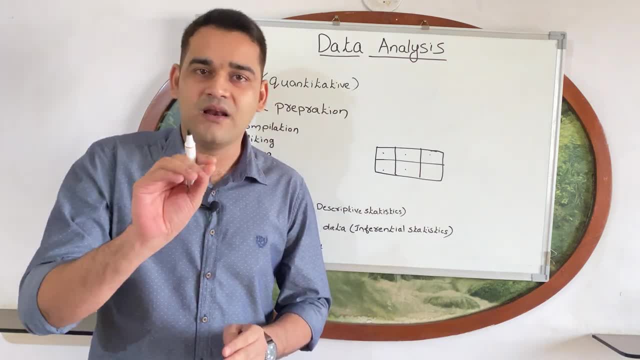 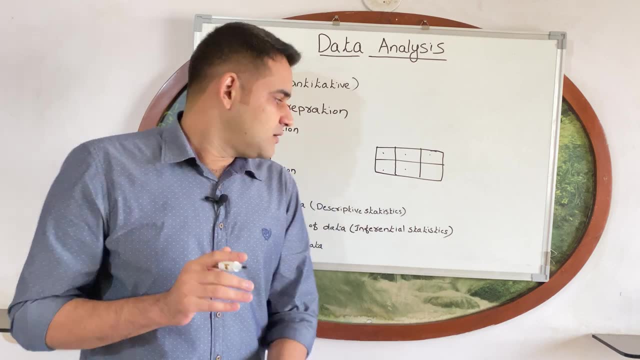 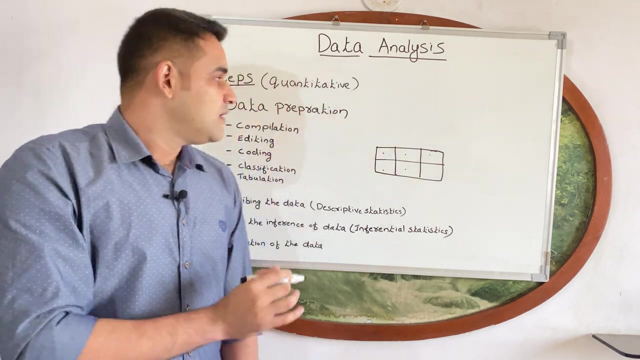 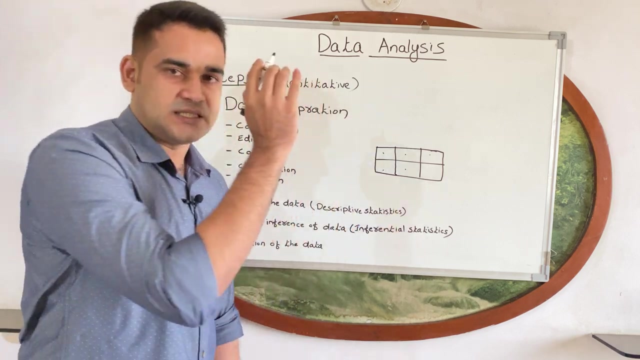 like that, in a column and in row, you will write it. that is tabulation. i am giving the example only. okay, that is tabulation. okay, that is regarding data preparation. next one is describing the data. the second step of data analysis is describing the data, or descriptive statistics. okay, in. 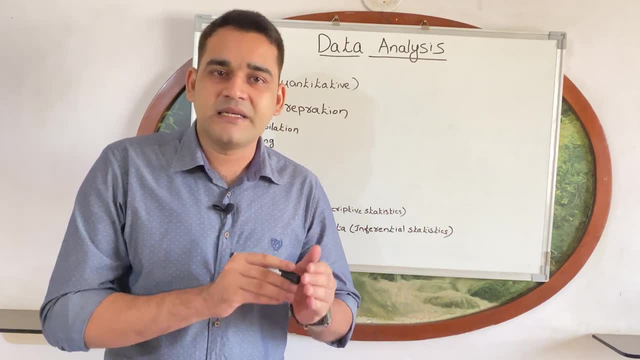 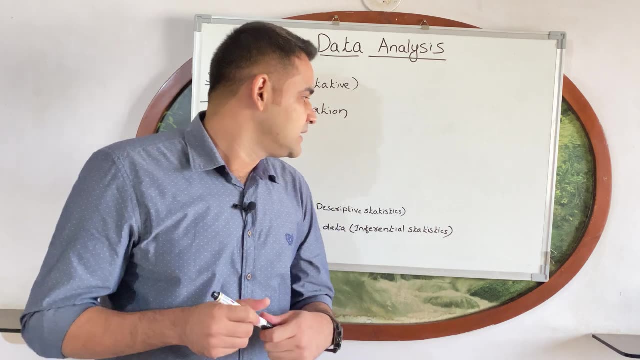 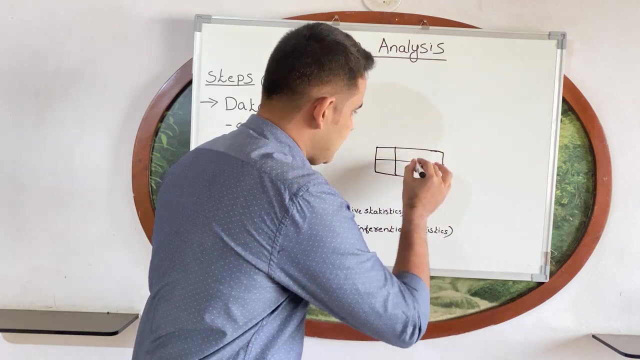 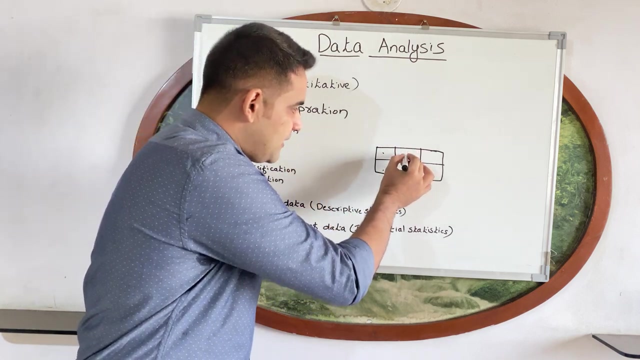 classified data in mathematical terms. In symbol you can call it as tables. In symbol you can call it as tables, That is, in rows as well as in columns. you can make, For example- I am just giving: This is tabulation- Here you can write male, female, their number of. 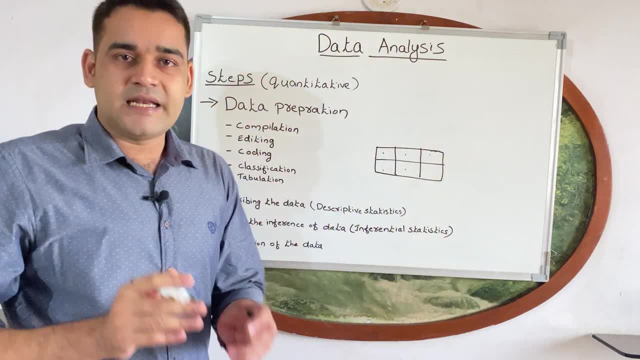 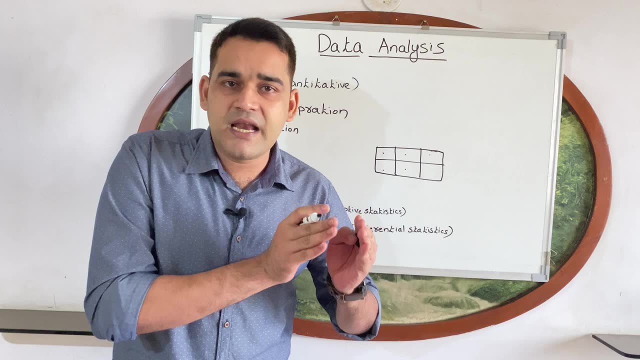 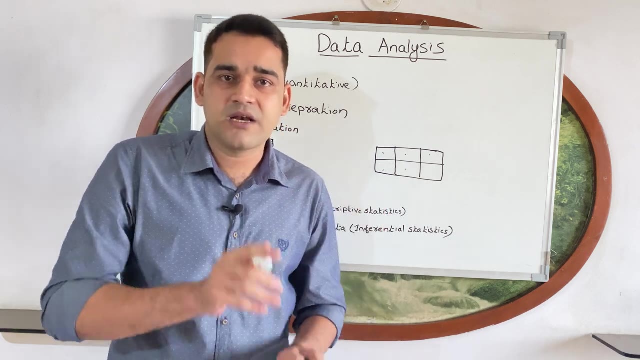 male and as well as number of females, their marks, like that tables you are making. That is tabulation. Tabulation means recording the classified data in mathematical terms. That is, using tables, that is, rows as well as in columns. In rows as well as in columns, you are. 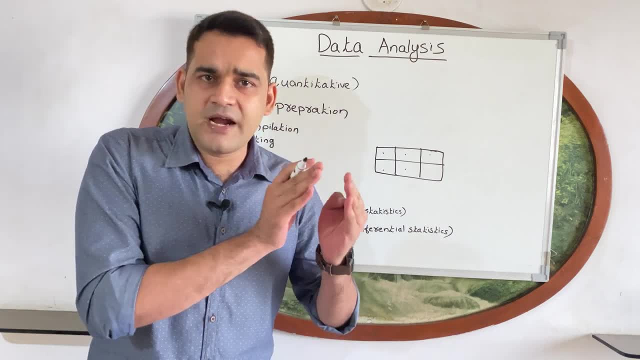 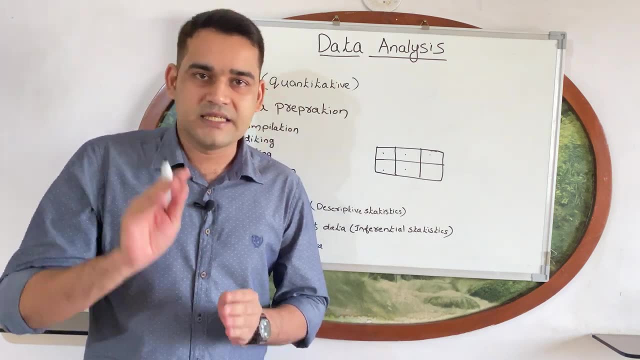 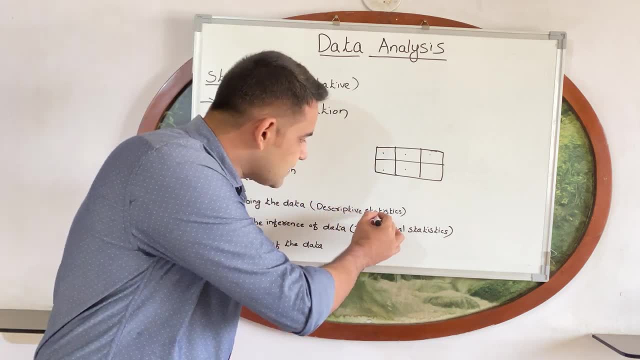 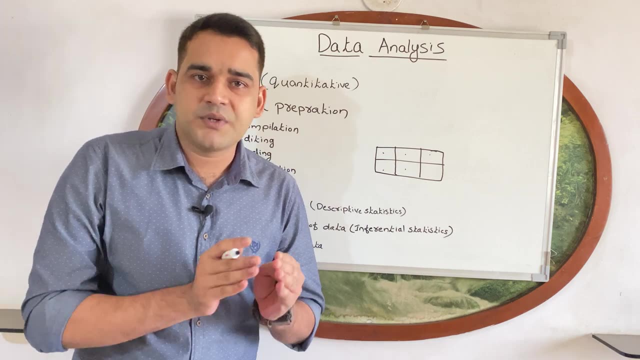 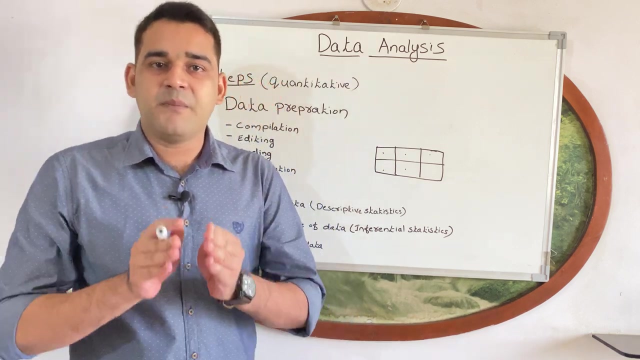 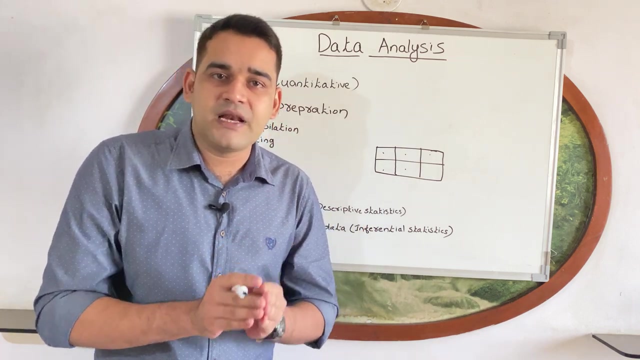 statistics. you learn in detail regarding what is descriptive statistics. okay, so here that is describing the data, or descriptive statistics means the researcher. in this step, the researcher will describe the basic features of the data, the basic features of the data, and the researcher will summarize a simple summary. okay, the researcher will make a simple. 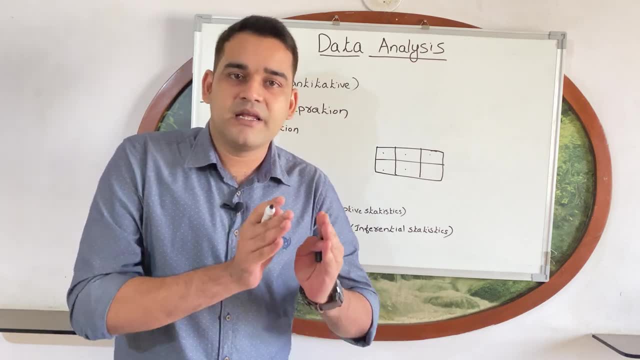 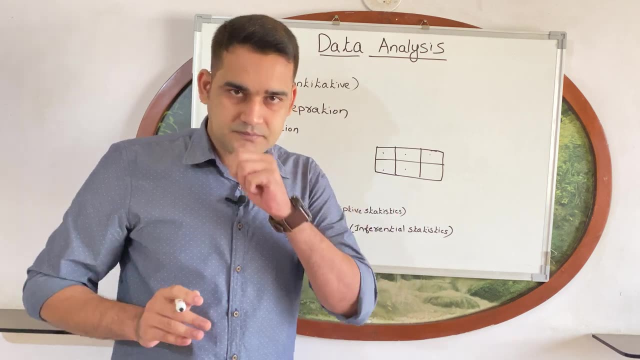 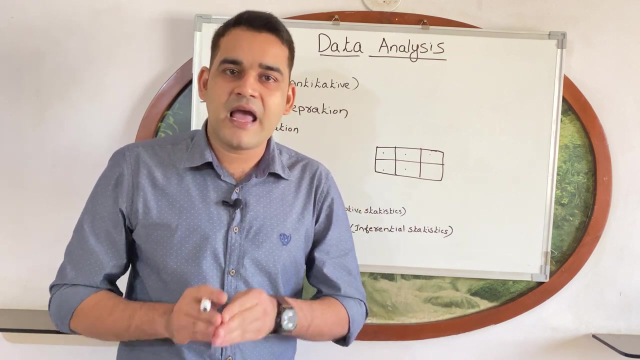 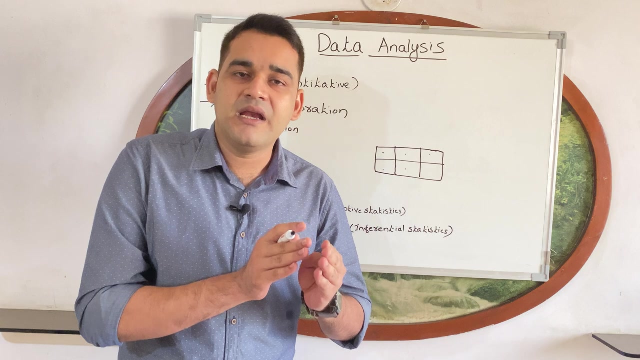 summary regarding the data, as well as the researcher will give or the researcher will describe a. regarding the basic features of the data: okay, for example, regarding the percentage of mark and regarding the average mark of the students in a particular class: okay, that is mean median mode range and standard deviation. that in 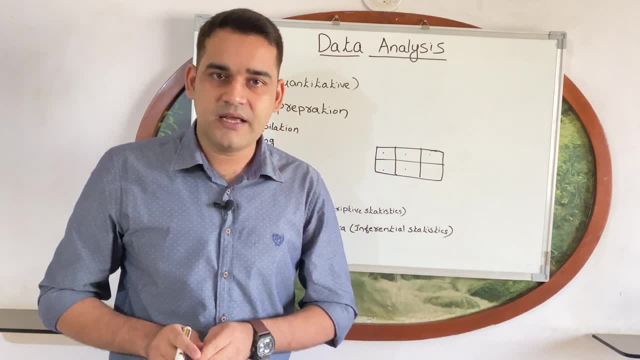 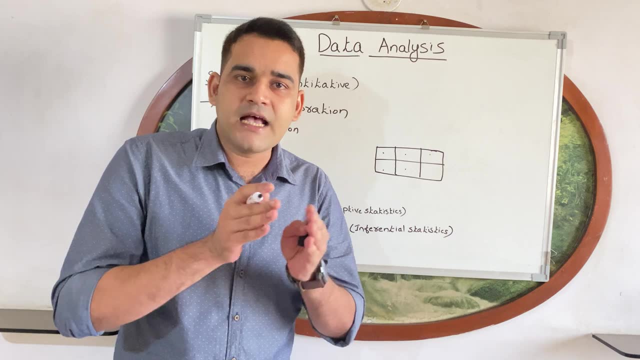 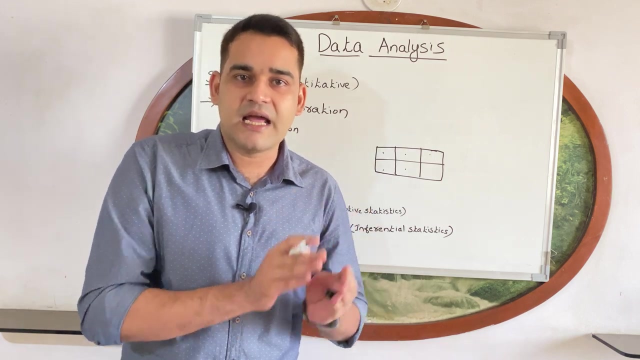 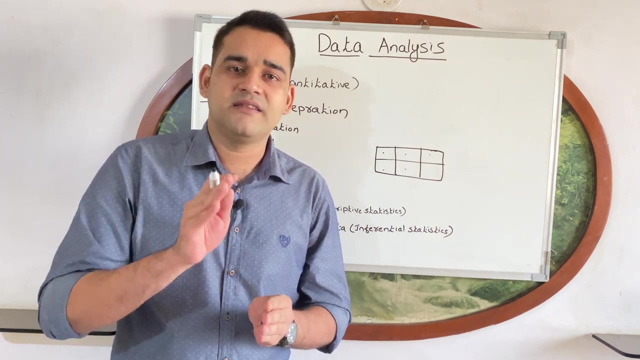 Statistics you will learn in detail. Okay, so describing the data means describing the basic features of the data as well as simply Summarizing the data. Okay, in a simple manner, the researcher will summarize the data regarding the percentage of the mark Regarding the average mark of the students, and all okay. So, regarding that, 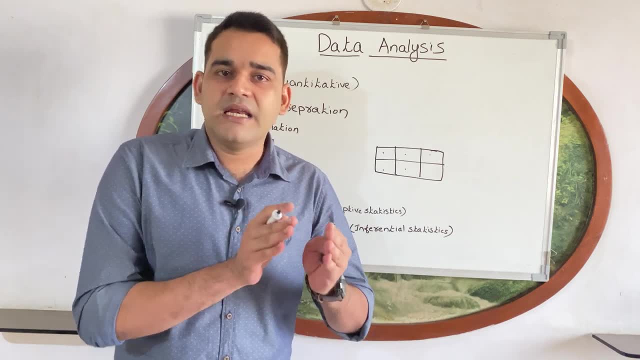 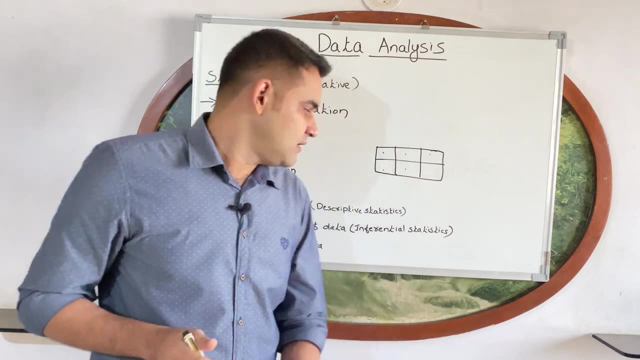 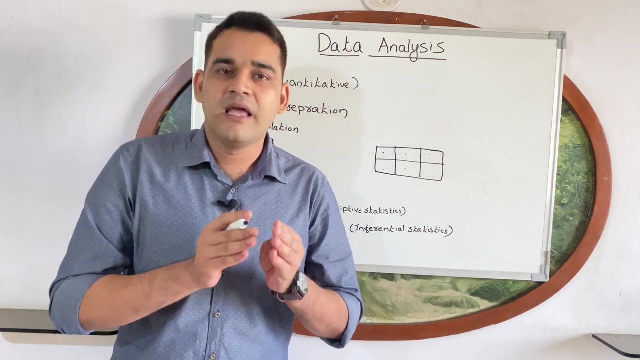 Regarding descriptive statistics, you learn in detail in statistics. Okay, Now you have to keep it in mind. regarding this, much point, only for data analysis. Next one is drawing the inference of data. Okay, drawing the inference of the data, or inferential statistics. It is also the part of the statistics, only. 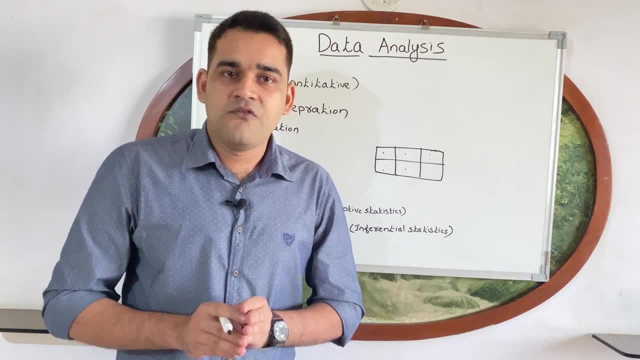 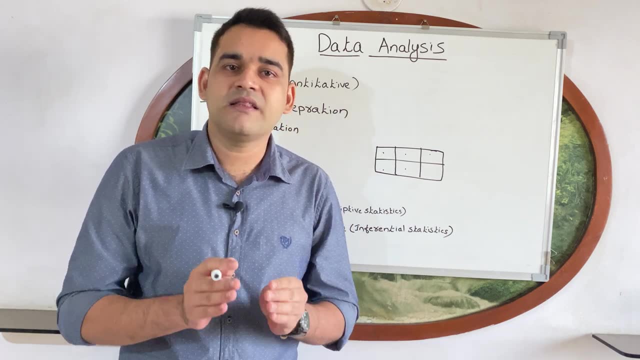 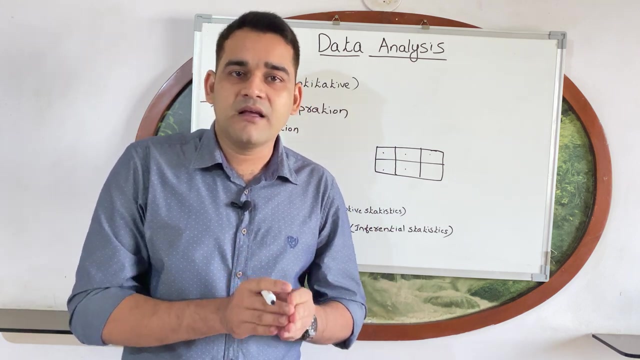 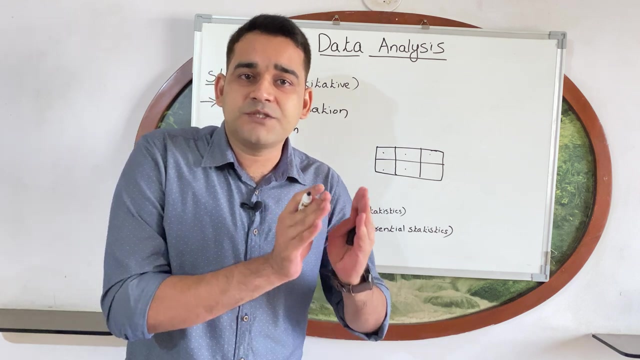 Okay, that is drawing the inference of the data, which means making the conclusion or the judgment of the data. Okay, making the judgment or the conclusion of the data, for example you want to know, regarding the relationship between the two things, or the Association between the two things or the difference between the two things, for example. 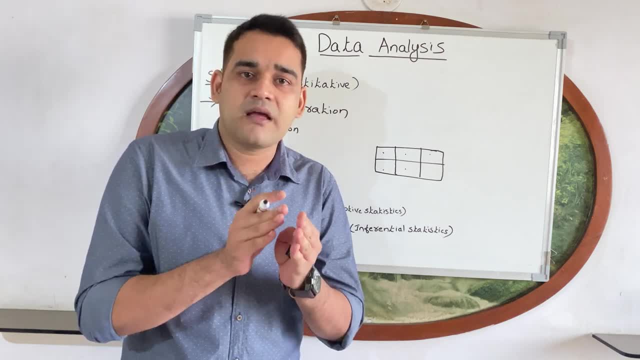 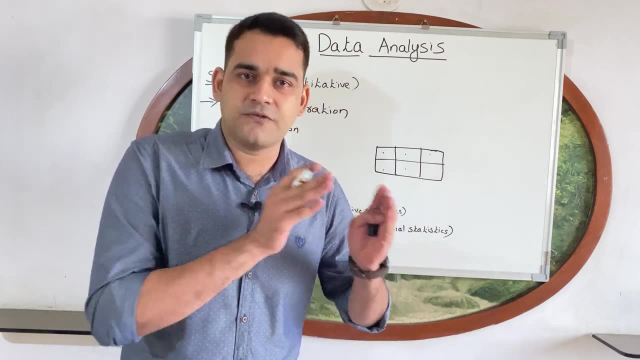 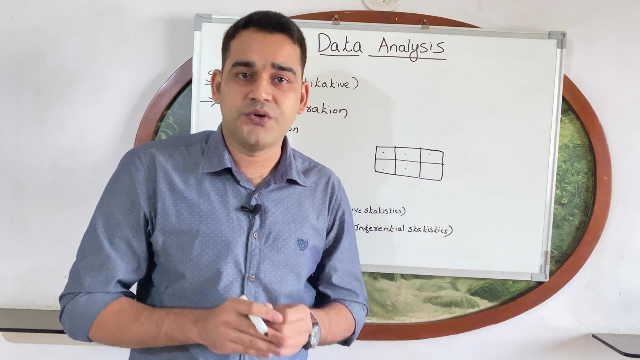 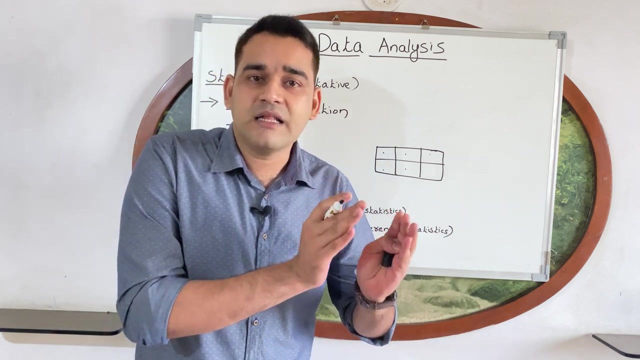 You want to know regarding the mark range or mark average between the male as well as the female students, as well as height and weight of the students. Okay, so in that the inferential statistics is used to know the relationship between the things, to know the Association between the things and to know the difference between the things. here you have to keep it in mind. 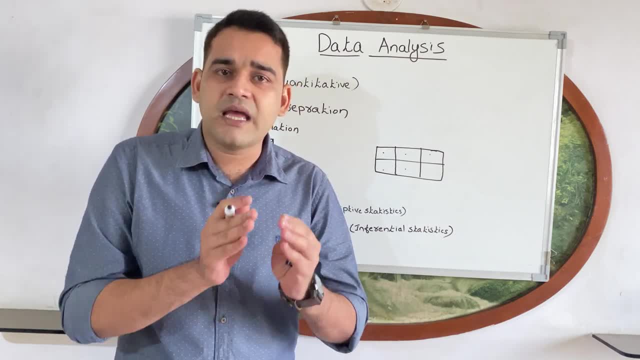 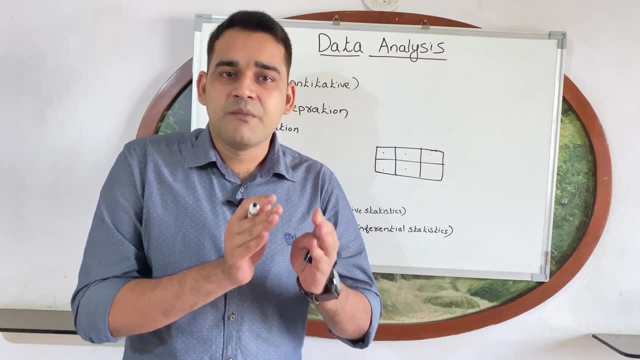 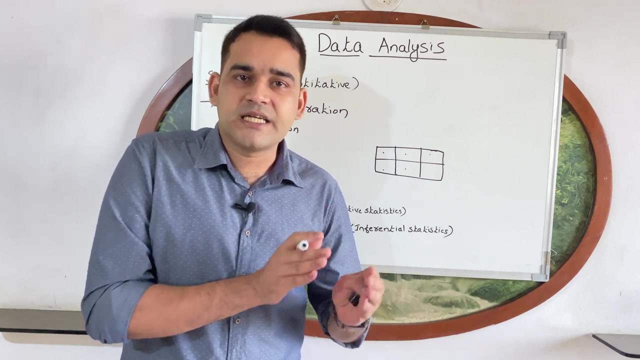 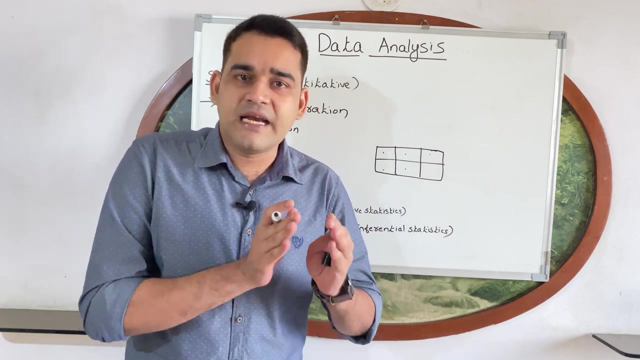 to draw or to make a conclusion and to make a Judgment is occurred in this step. Okay, so drawing inference means making a conclusion and Judgment, and it will help you identify regarding the association, Regarding the relationship and regarding the difference between the things. Okay, mainly t-test, as well as ANOVA and other use in inferential statistics, That is. 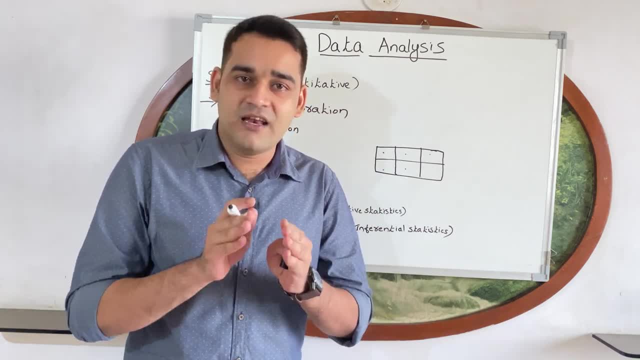 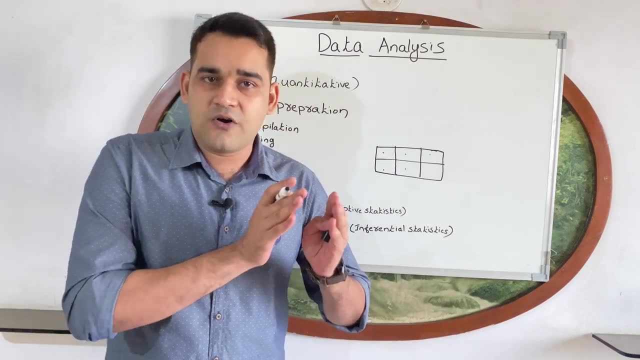 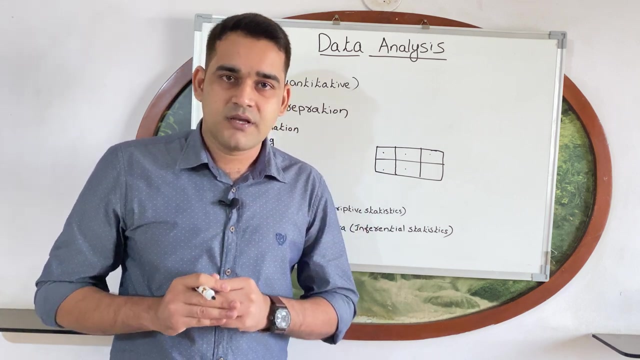 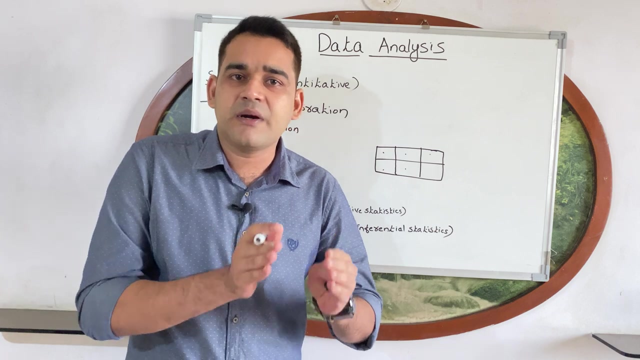 inferential statistics. you will learn in detail in Statistics. okay, and the last step is interpretation of the data. okay, interpretation of the data. So what is mean by interpretation of the data? interpretation of the data means If you got the result. okay, after analysis, you got the result in interpretation of the data. 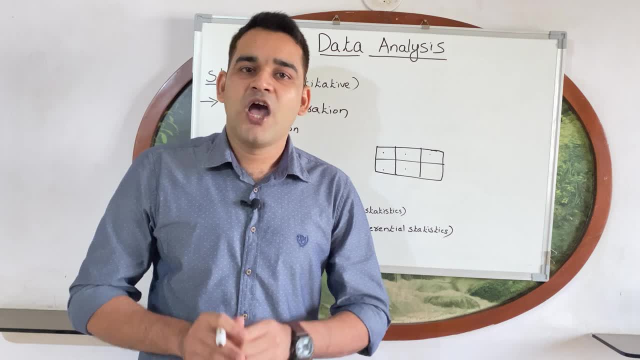 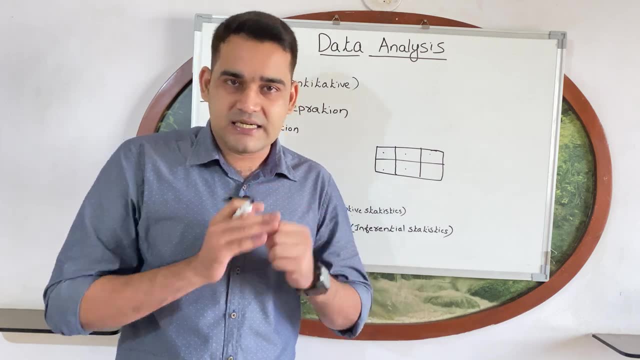 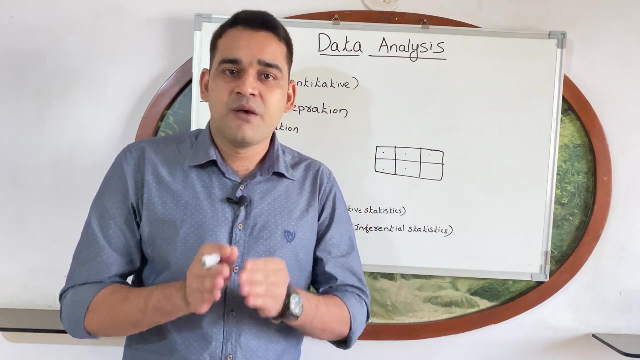 You will do the critical examination- Okay, you will do the deep Examination regarding that result and you will explain the result. Okay, you will explain the result. Explaining the result, as well as making that result in an understandable manner, Making the sense of the result, is called. 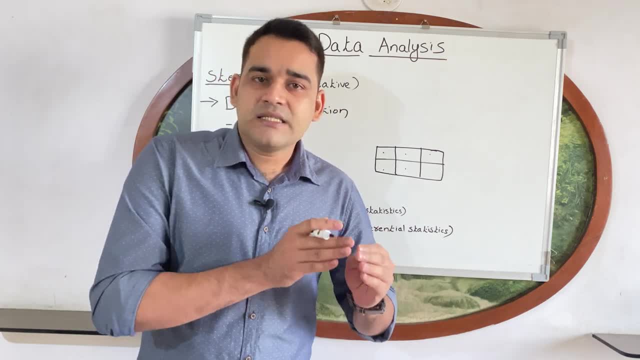 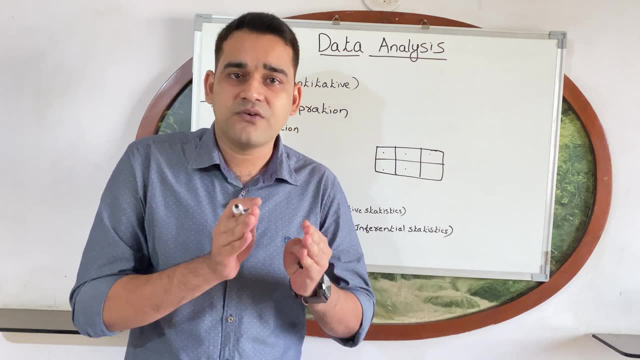 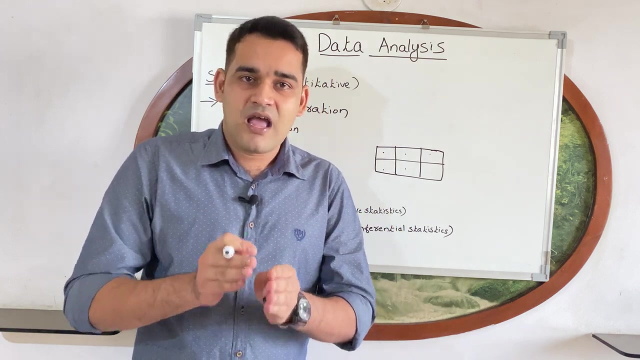 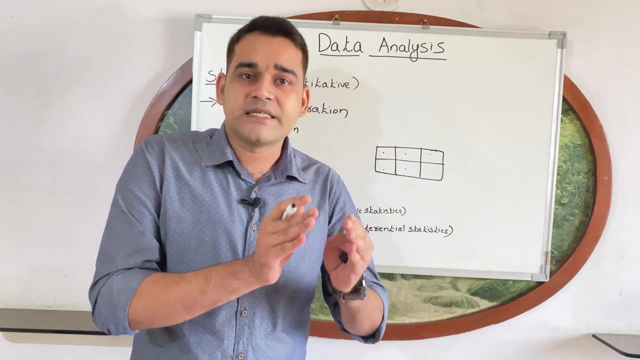 interpretation of the data. Okay, so in analysis of data you got the result and finally, in that result, in interpretation of data, what you are doing you are doing a critical examination deeply, you are examining that result and you are making an explanation regarding that result And you are making a sense of that answer that is in a understandable manner. 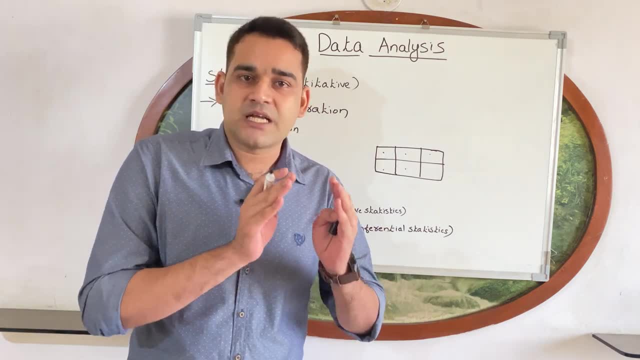 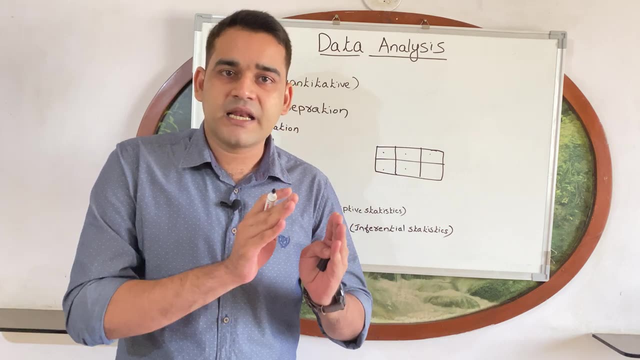 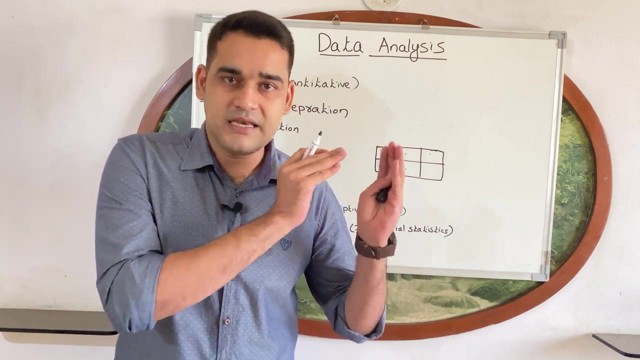 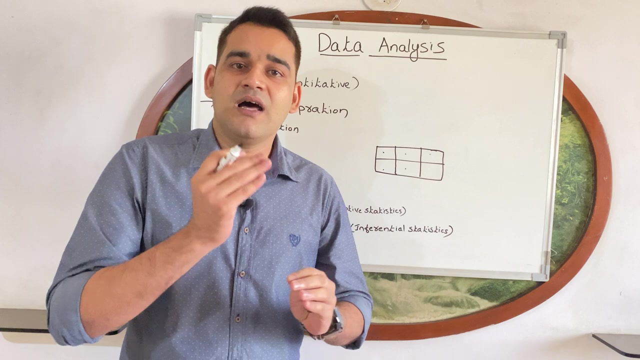 For example, in the mark sheet regarding different subjects. regarding different subject, the marks of the students. for example, in anatomy, for theory, how much mark that student got, and regarding the practical and regarding the internal assessment and the total mark. like that, in a proper order, it is used to show the.